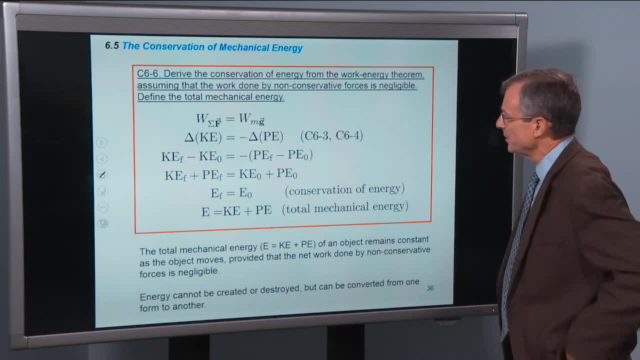 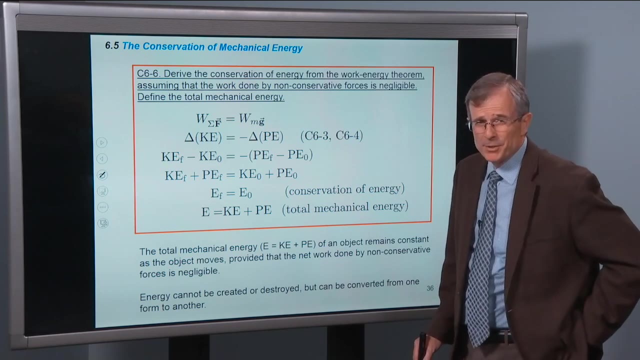 Derive the conservation of energy from the work energy theorem. assuming that the work done by non-conservative forces is negligible, Find the total mechanical energy. Alright, so we're going to do a derivation here And I expect you to be able to work through this one. It's an important one. 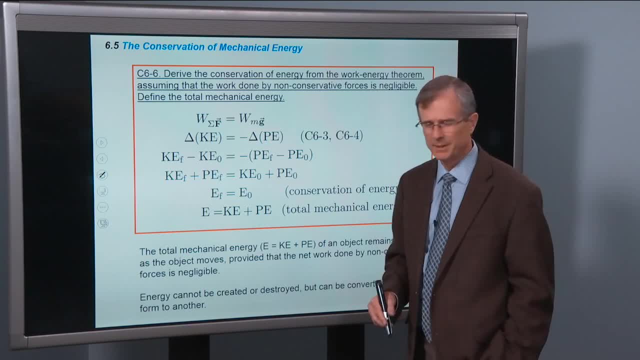 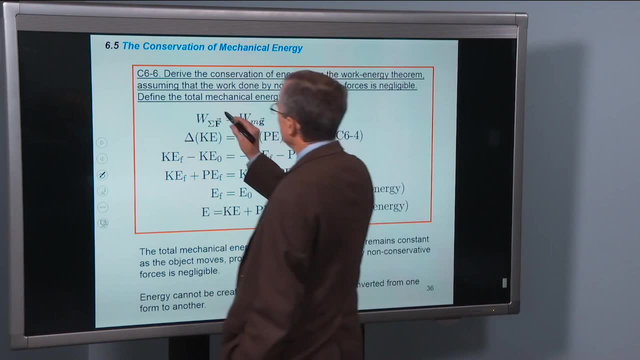 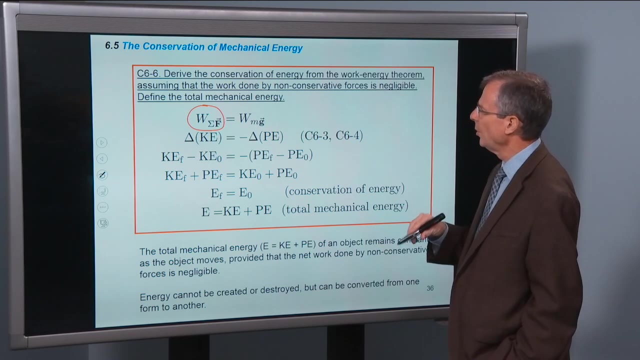 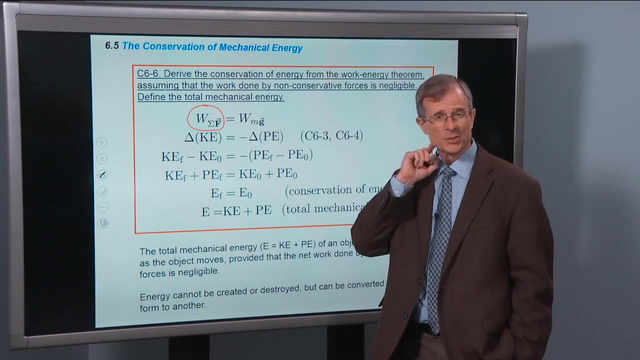 It is based entirely on concepts we've already done. It's quite easy and straightforward. So the work done by the net force We're going to consider, only the work done by conservative forces. The only one that we've considered so far is gravity. 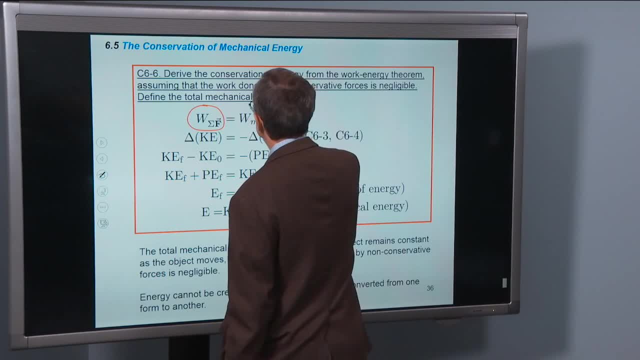 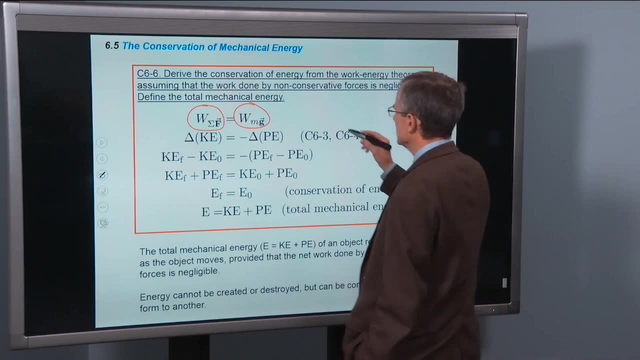 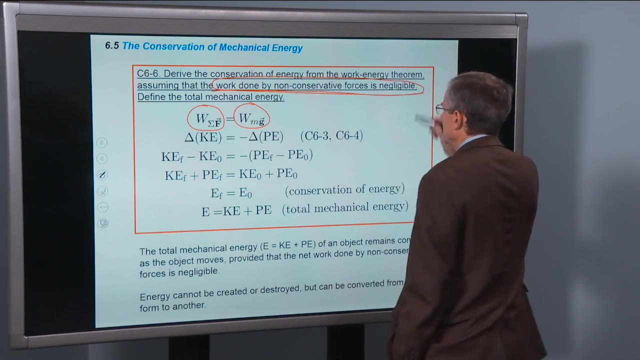 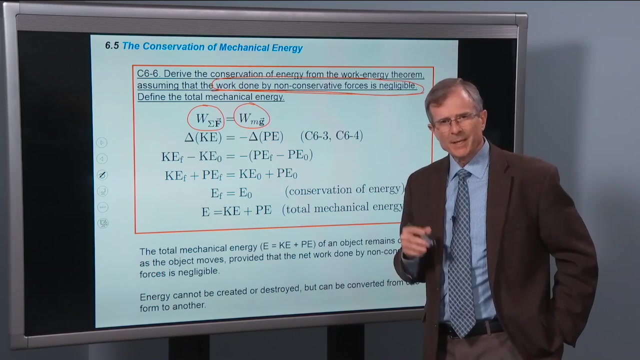 So let's just put gravity in by itself And we're assuming that the work done by non-conservative forces is negligible. Now, this is a mouthful, But it's an important mouthful. We have to be able to assume that the work done by non-conservative forces is negligible. 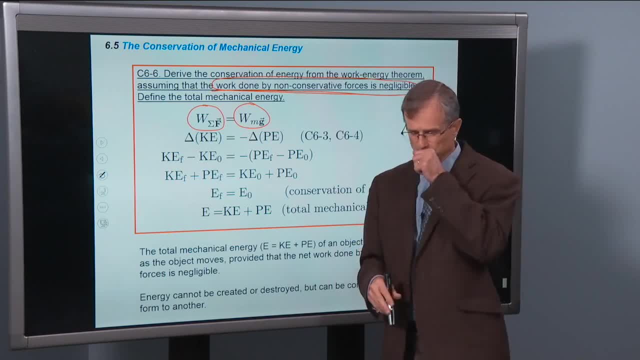 What about friction? Kinetic friction? That's certainly one that we have to worry about. Air drag. If we can ignore the work done by those types of forces, then energy is conserved. So we're ignoring here the work done by friction. 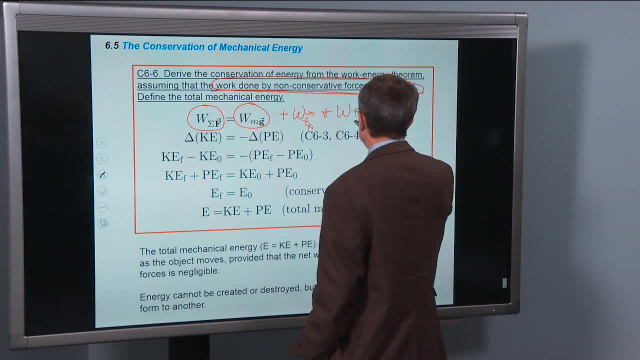 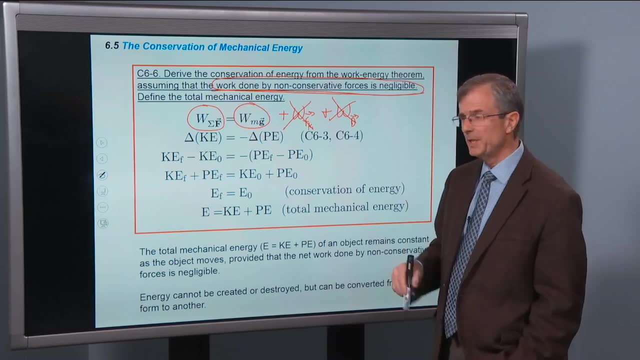 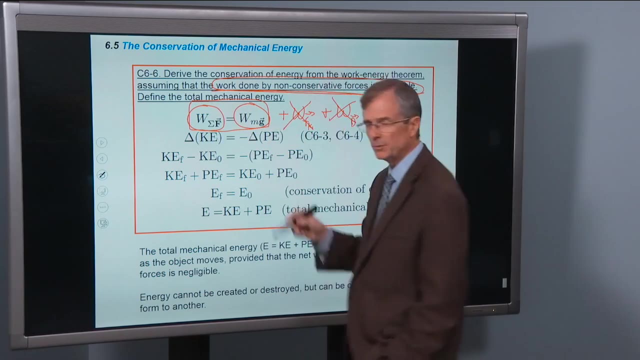 for example, or the work done by drag. So we're considering these to be negligible, meaning we can neglect them in the analysis, And so all we're left with is: the work done by the net force is equal to the work done by gravity. 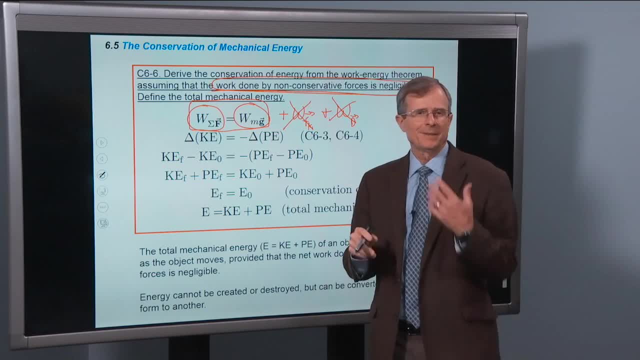 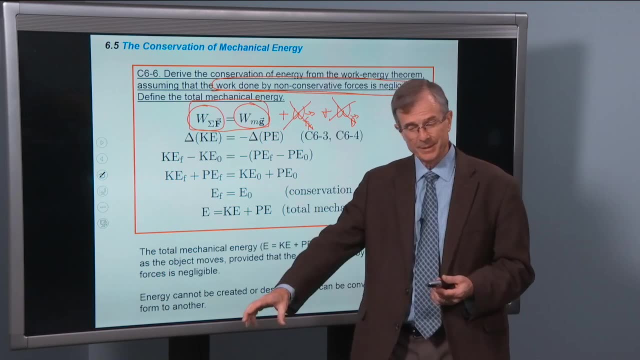 One instance of where you couldn't neglect friction would be the case of the block moving along the tabletop that I did in the demo video. Well, that friction was doing a lot of work and it's not going to be negligible in that case. 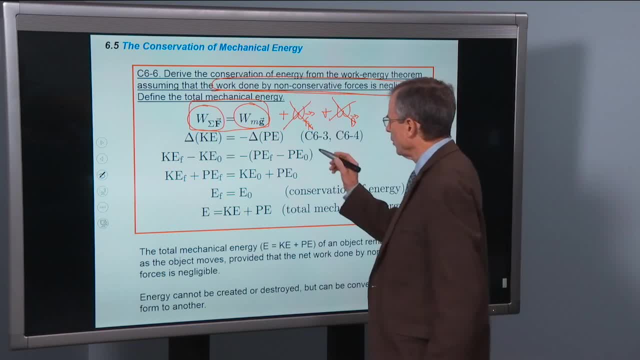 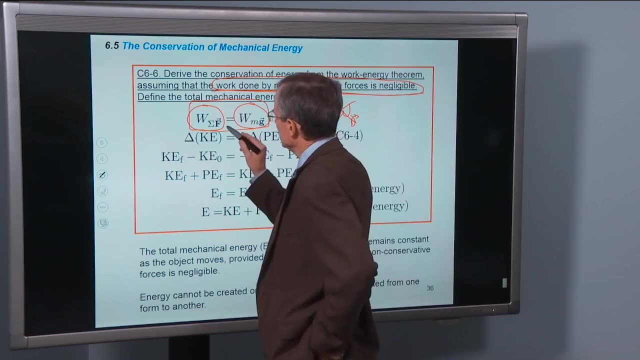 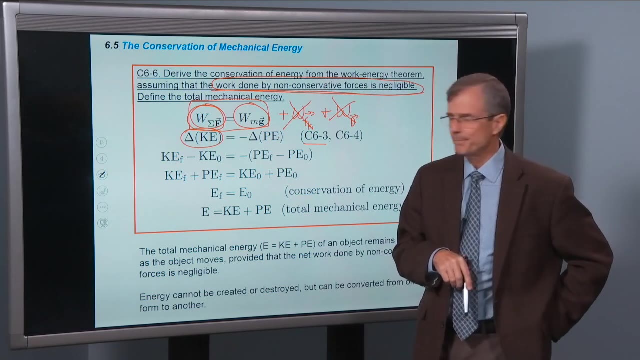 Alright, Now what we'll do is invoke concept C6-3, the work energy theorem, to set the work done by the net force equal to the change in the kinetic energy. That's the work energy theorem, And we're going to use the concept C6-4. 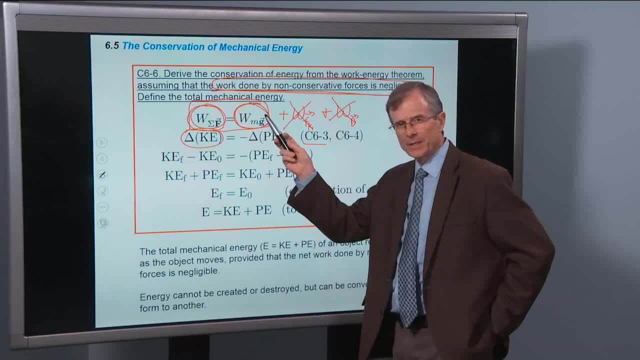 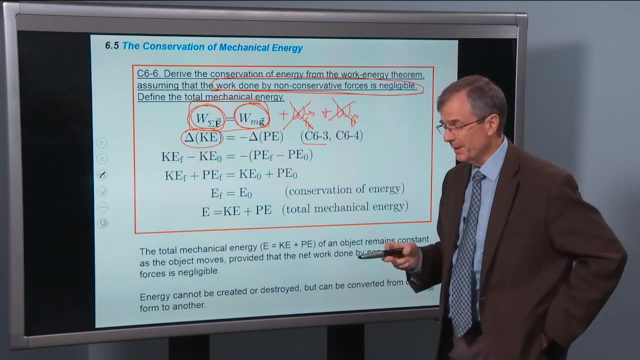 that the work done by gravity is the negative of the change in the gravitational potential energy. So those two concepts get us pretty much the rest. The rest of it is just algebra. It's not that hard. Change in kinetic energy is the final minus the initial. 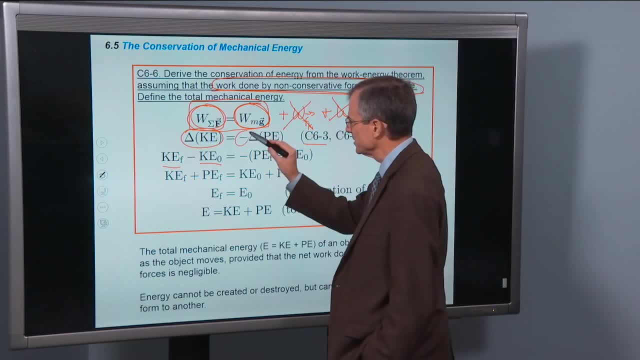 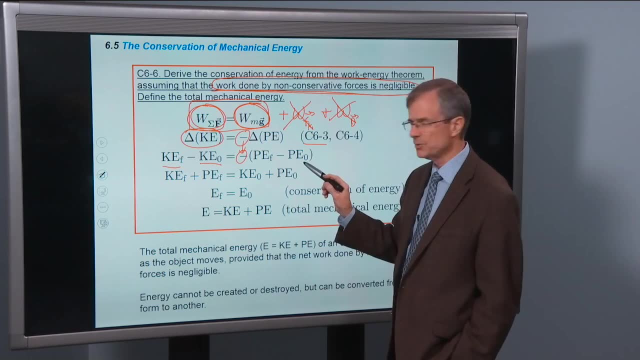 No problem there. The change in the potential energy, this minus sign, just comes along for the ride. The change in the potential energy is the final potential energy minus the initial potential energy. Now what we're going to do is to try and collect terms on the same side of the equation. 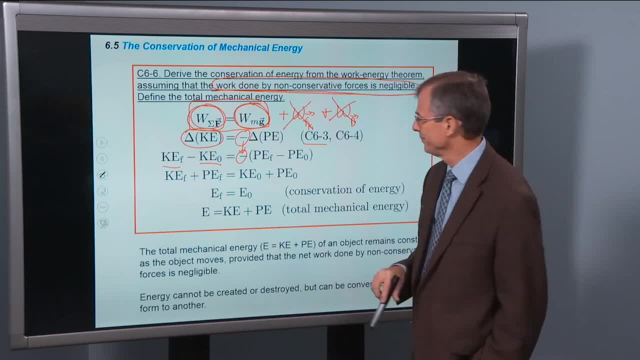 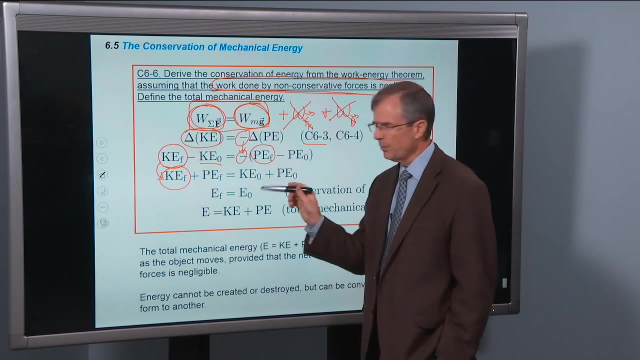 that refer to the final time. So here's this final kinetic energy. It just comes along for the ride. It stays on the left-hand side of the equation. Well, here's a term that involves the final potential energy. I want to get it on the left side of the equation. 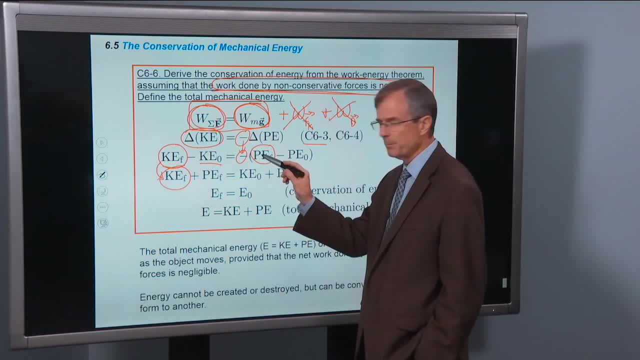 How do I do that? Well, it's here on the right side with the minus sign in front of it, So I can add the final potential energy to both sides of the equation. It'll cancel on the right side and appear on the left side. 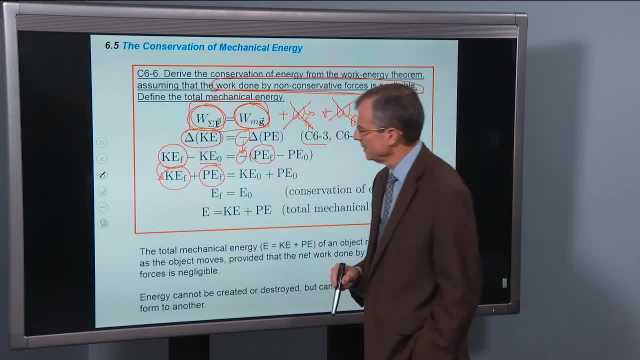 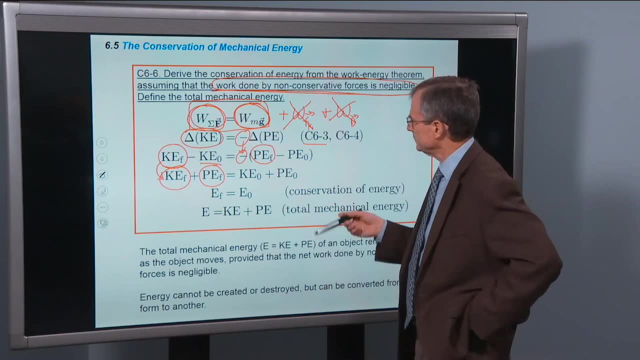 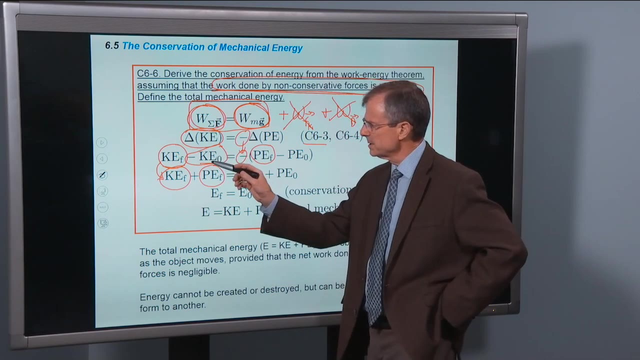 And here it is. Here's its appearance. Now, on the right side, I'd like to collect all the terms involving the initial time. Here's a term involving the initial time Minus the initial kinetic energy, If I want it on the right side of the equation. 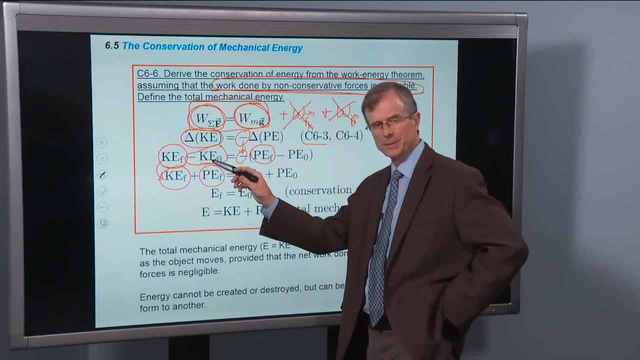 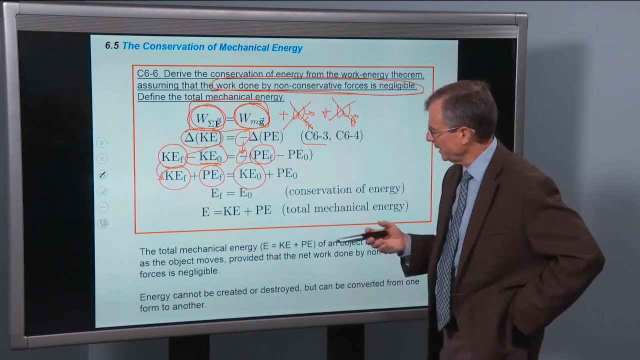 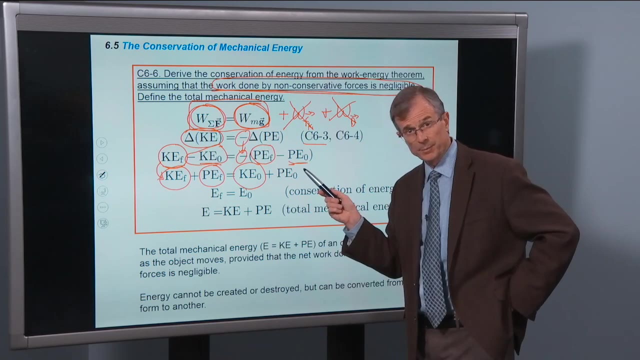 I'm going to add it to both sides of the equation. It'll cancel on the left side and appear on the right side, right here, And then finally we've got this term that is, a negative-negative initial potential energy Negative times. negative is positive. 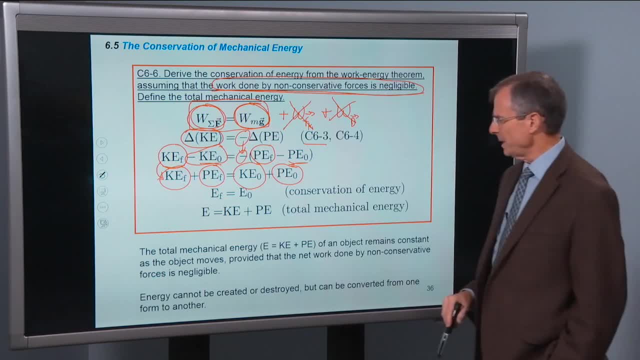 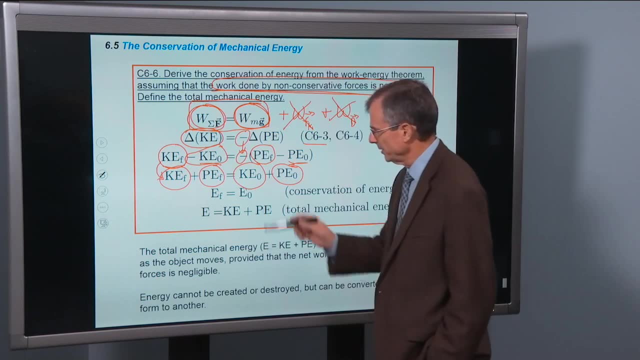 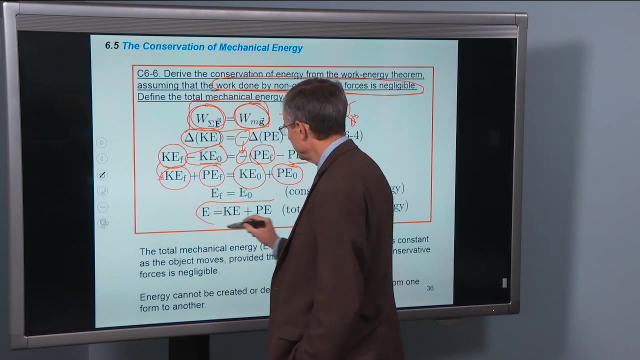 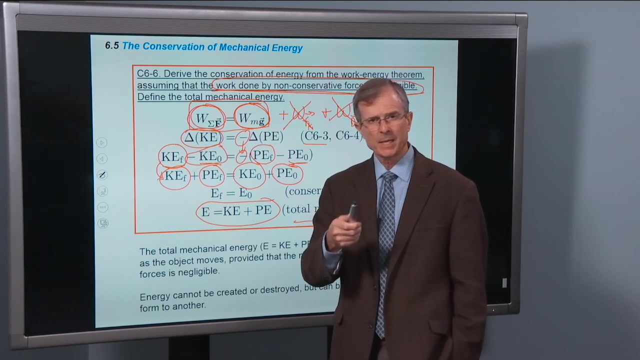 So here it is. So what we have here is a rather curious thing. I've got the final kinetic plus the final potential on the left, the initial kinetic plus the initial potential on the right. So we define the total mechanical energy as the sum you add up the kinetic plus the potential. 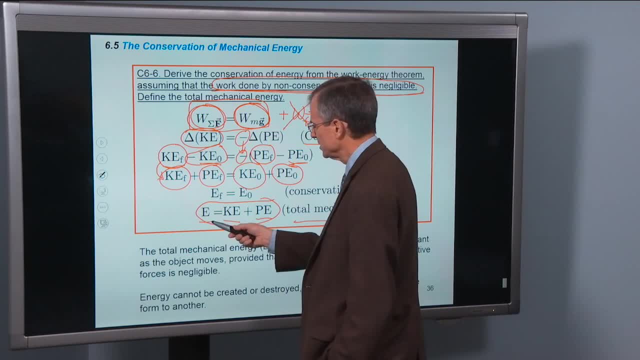 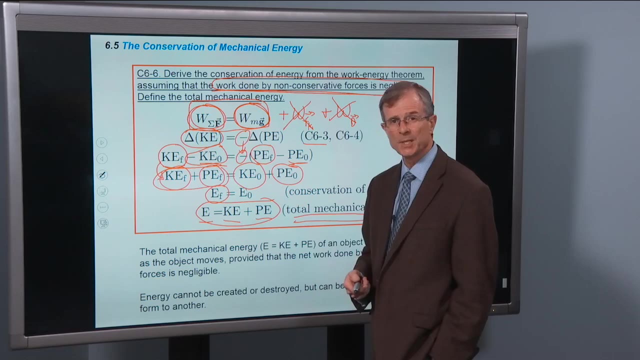 Kinetic energy plus potential energy is called the total mechanical energy. With that definition, then, the left side of this equation is the final kinetic plus final potential. That's just the final total mechanical energy, And on the right side we have the initial kinetic plus initial potential. 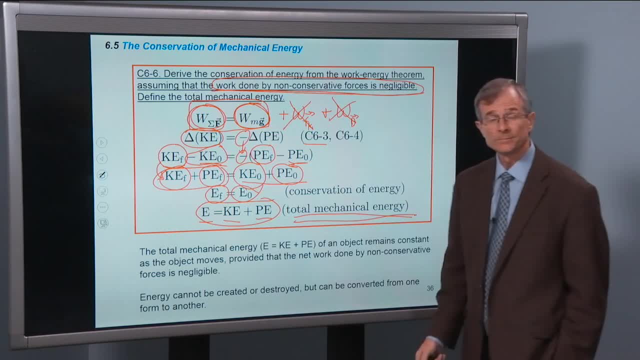 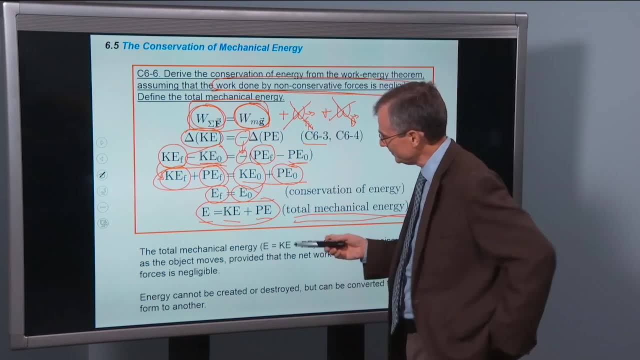 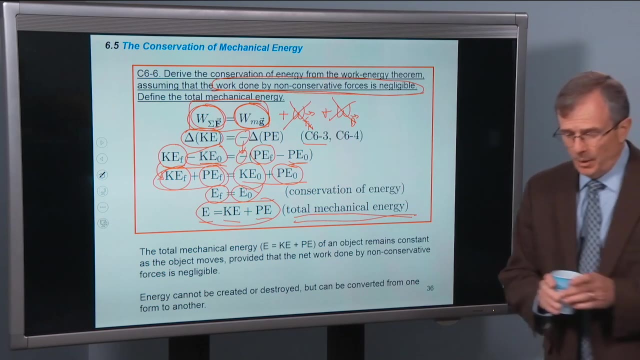 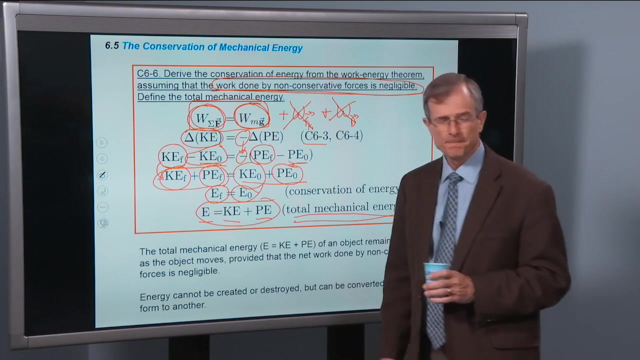 That's just the initial total mechanical energy. So what this says is pretty cool: The final total mechanical energy Equals the initial total mechanical energy. It's pretty amazing And this is very, very useful in problem solving, And I'll do a couple of examples. 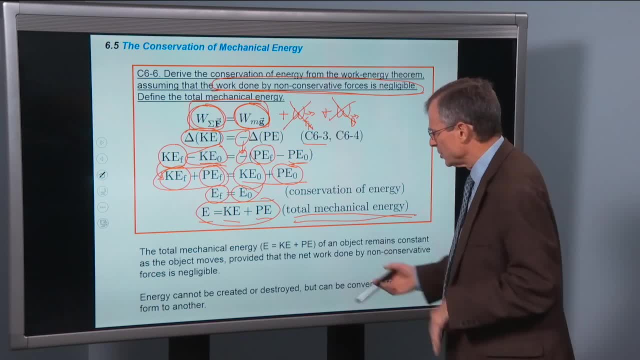 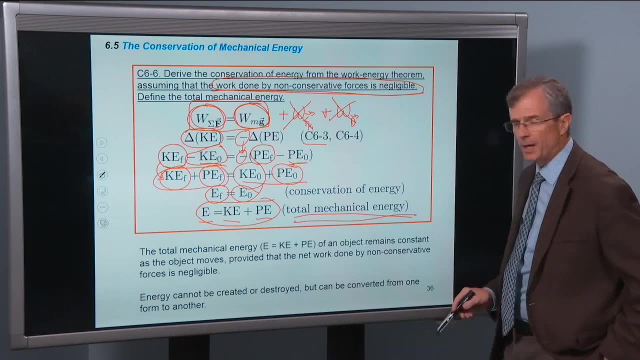 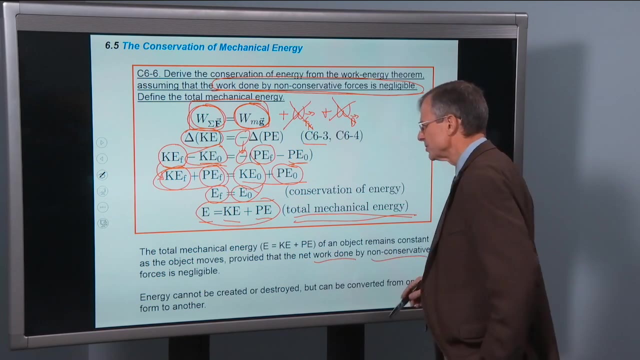 But first a couple of statements about this. The total mechanical energy E equals kinetic plus potential of an object remains constant as the object moves around through space, Provided that the work done by non-conservative forces is negligible. So you have to be able to ignore. 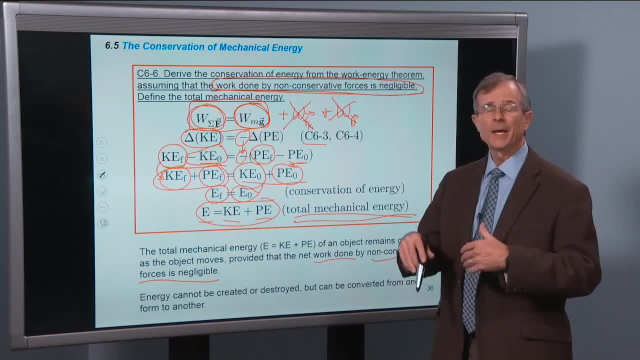 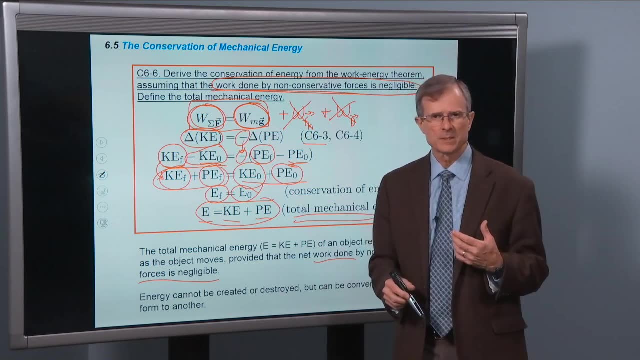 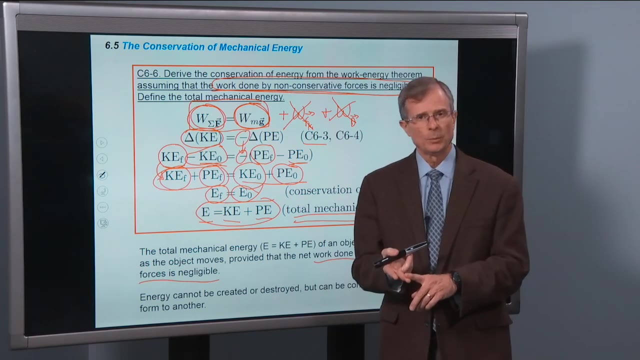 those non-conservative forces, Then you'll get conservation of energy. Now, this is the first example of a conservation principle that we'll talk about in this class. We will later talk about the conservation of momentum and the conservation of angular momentum. But when physicists say that a quantity is conserved, 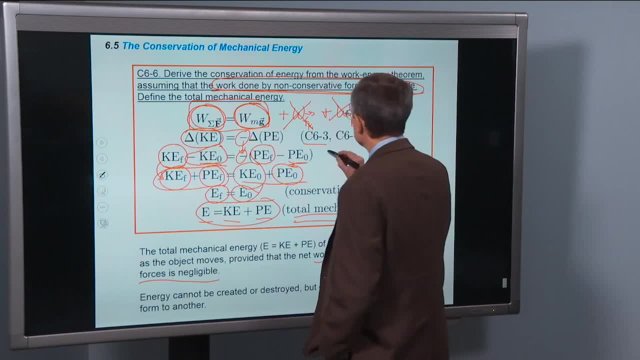 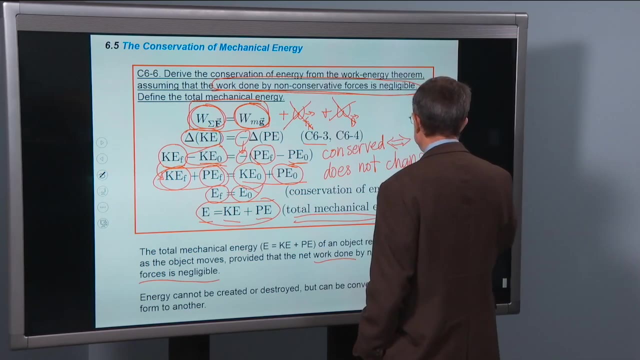 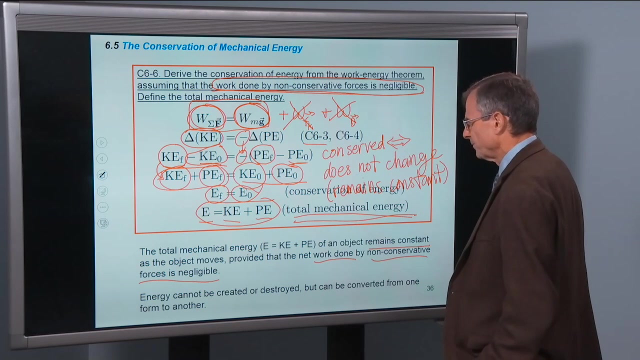 what they mean is that it does not change. So conserved means that it does not change. That's what we've said here. It remains constant. So if I say that energy is conserved, I mean it remains constant as the object moves through space. 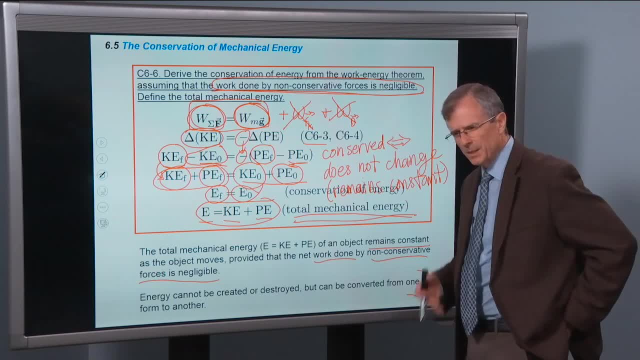 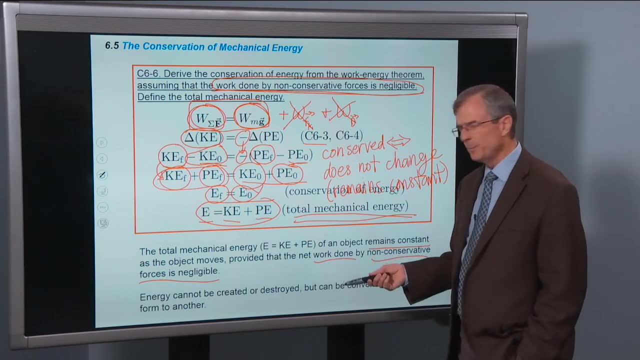 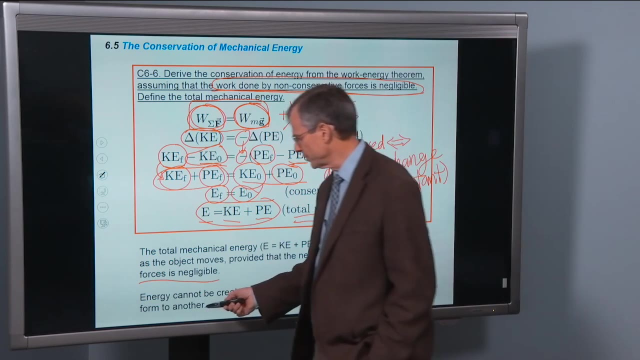 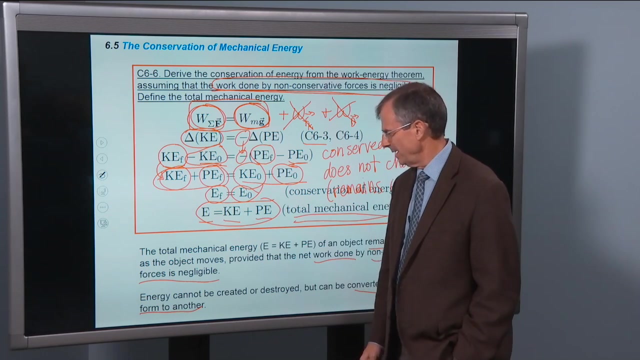 And here's the kind of more, a little deeper philosophical statement of the conservation of energy. Energy cannot be created or destroyed, But it can be converted from one form to another. So we can convert kinetic to potential or potential back to kinetic, But the energy, the total energy. 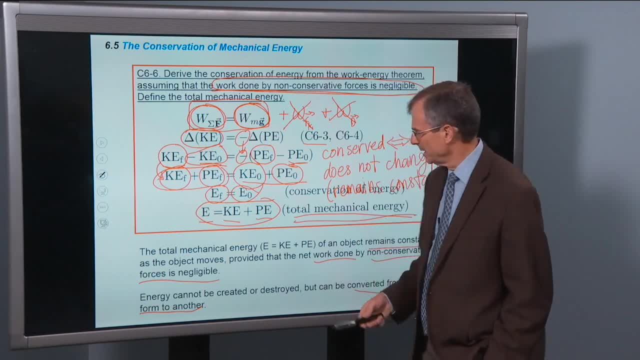 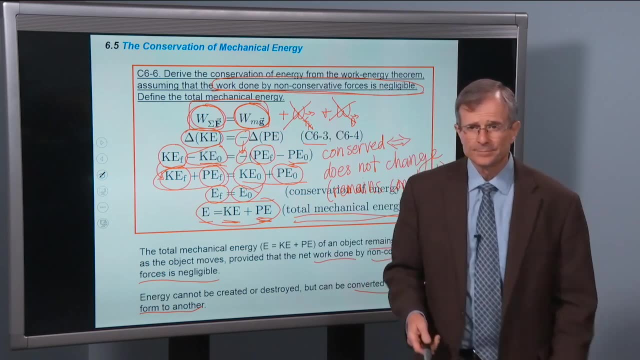 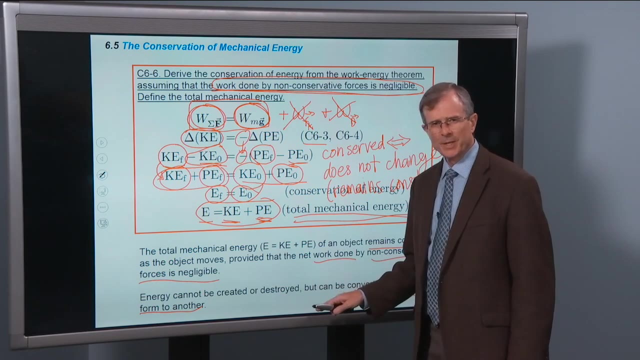 the sum of the two has to remain the same. So if you increase the potential energy, you're going to have to decrease the kinetic energy, or vice versa. We'll see this in a moment, This in various guises during this semester, when we talk about springs. 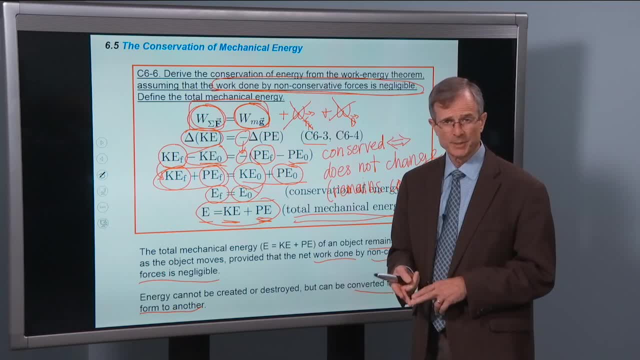 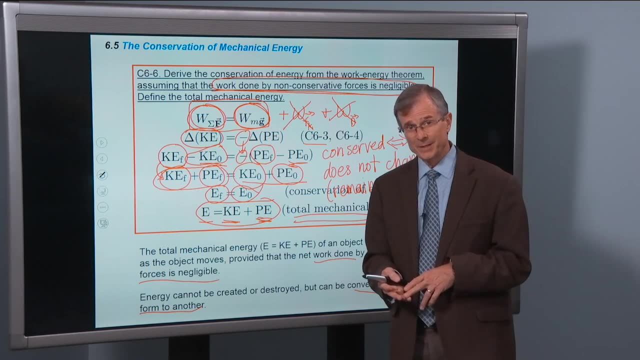 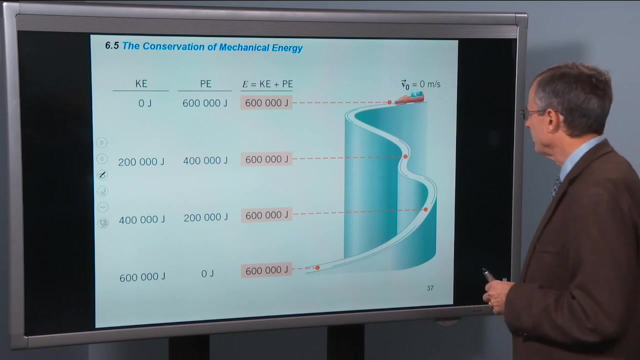 and also next semester when we talk about electric potential energy, and also next semester when we talk about E equals mc. squared that energy and matter are different forms of the same quantity and through Einstein's famous relationship. So here's an example: You've got a sled. 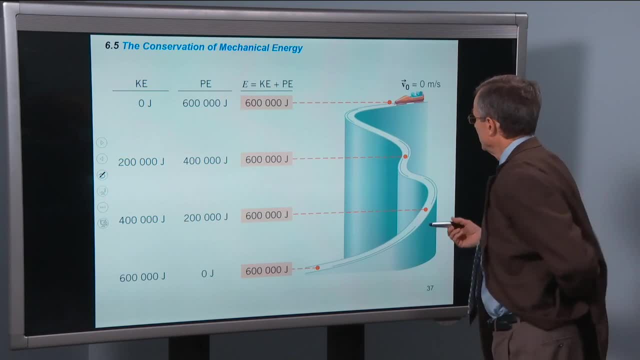 Suppose you consider it to be frictionless- that slides down this track At the top. when it's at the top of the track, the height is large, And so the gravitational potential energy must also be large. So we're going to start off with a lot of 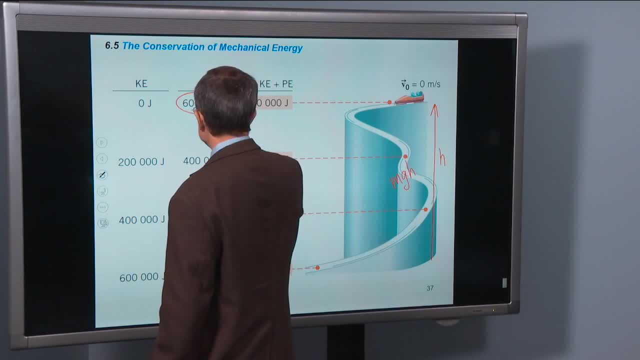 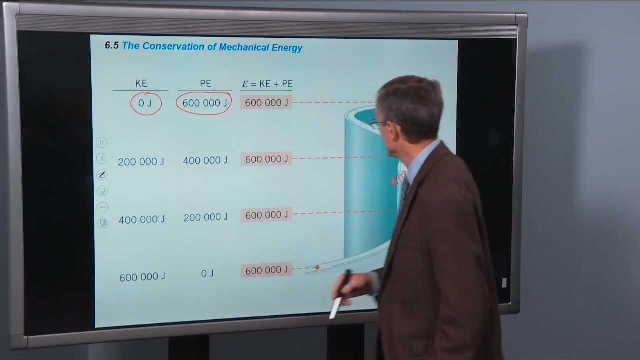 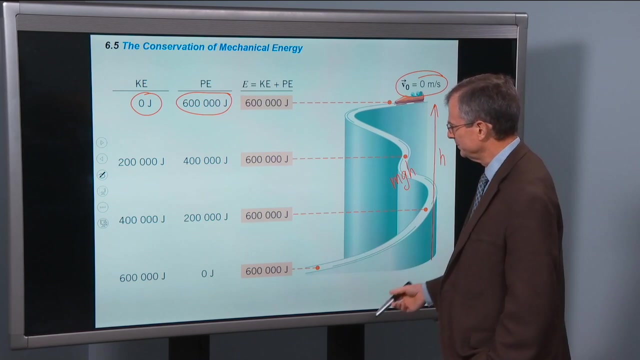 gravitational potential energy, So maybe 600,000 joules, when it's at this top position. The kinetic energy at the top is zero, because we're releasing it from rest. So then it goes down the track in the middle. here somewhere It still has some gravitational potential energy. 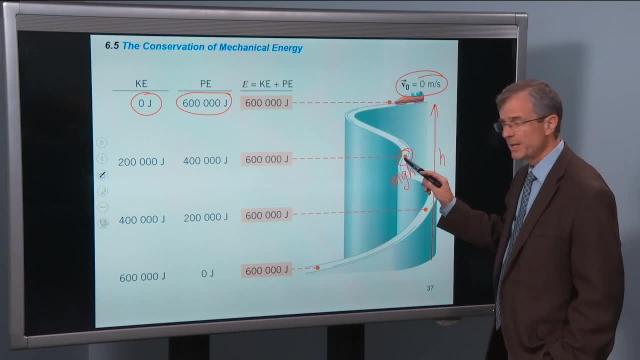 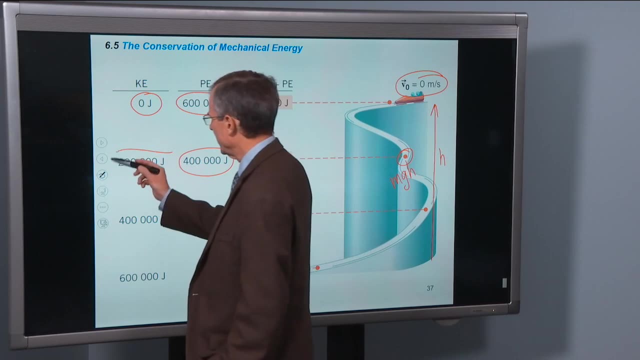 but it's less. It has less potential energy than it did before, So 400,000 instead of 600,000.. But it's gained some kinetic energy, so that the sum of the two, 200,000 plus 400,000, is still 600,000. 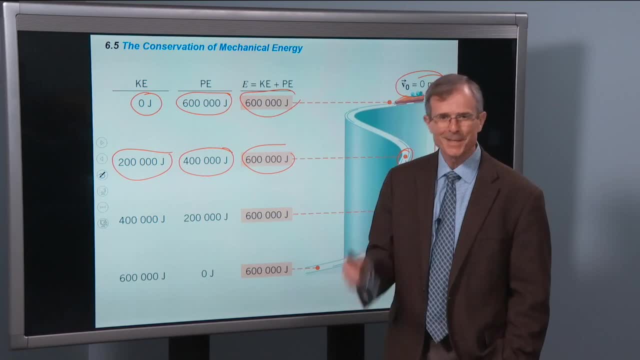 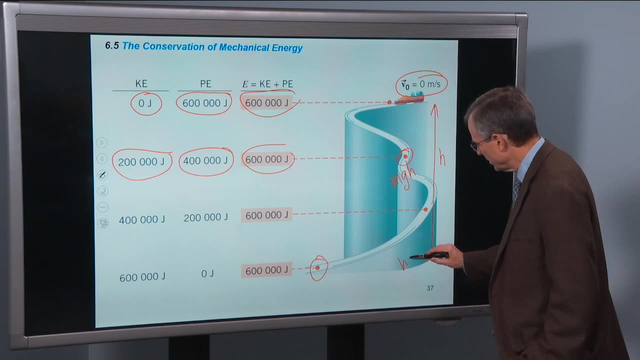 That's what we mean by a conserved quantity. It's constant, It doesn't change. And then now down here at the bottom, where h equals zero, mgh must also be zero And the gravitational potential energy is zero. But now, if energy is conserved? 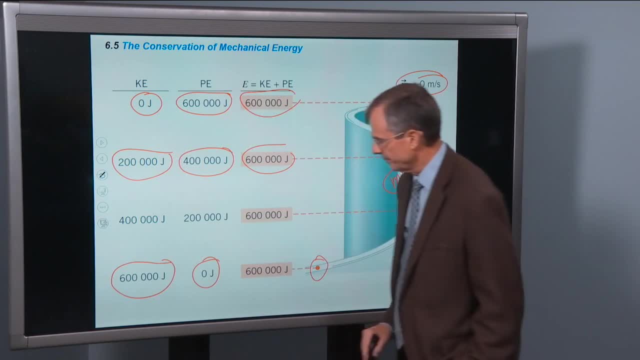 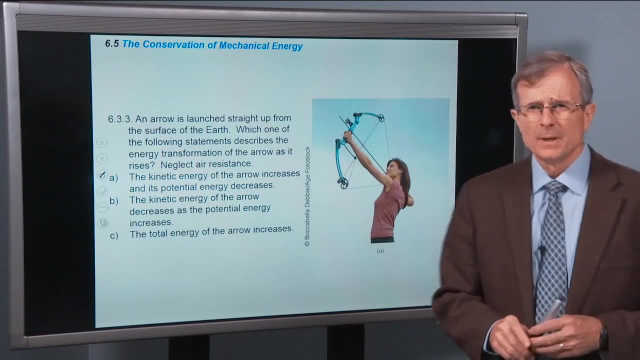 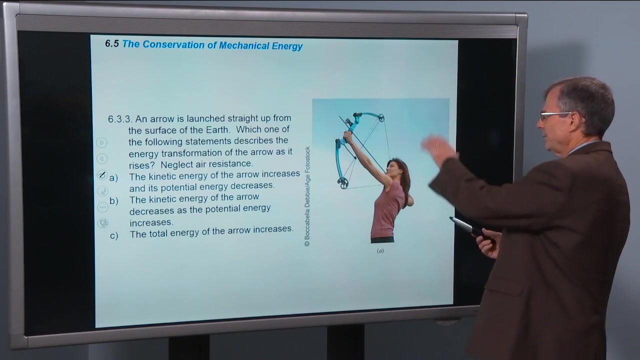 then, lo and behold, that energy is completely contained in kinetic energy. Let's do an example: An arrow is launched straight up from the surface of the earth, So we actually have to have the arrow shoot straight up to be this example, which one of the following statements describes: 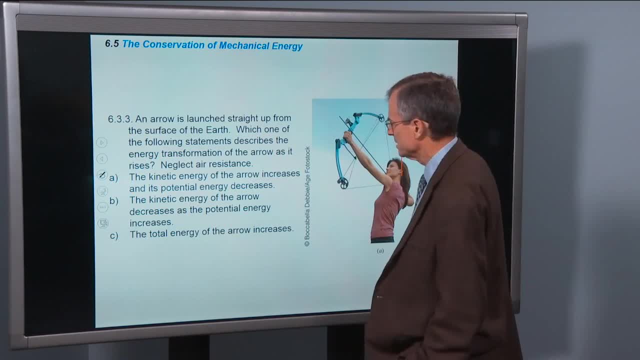 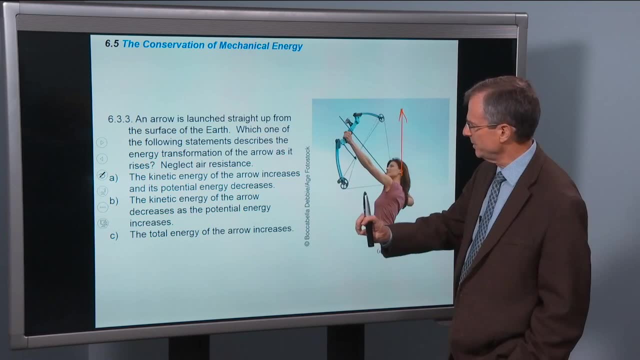 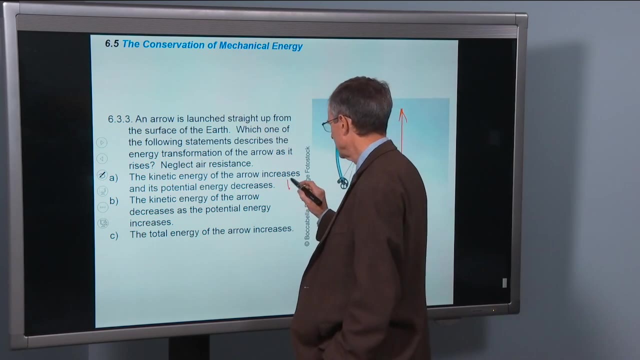 the energy transformation of the arrow as it rises, Neglect air resistance. So as it's rising up, the kinetic energy of the arrow increases and its potential energy decreases. True or false? That's not true, Because as you get higher and higher, 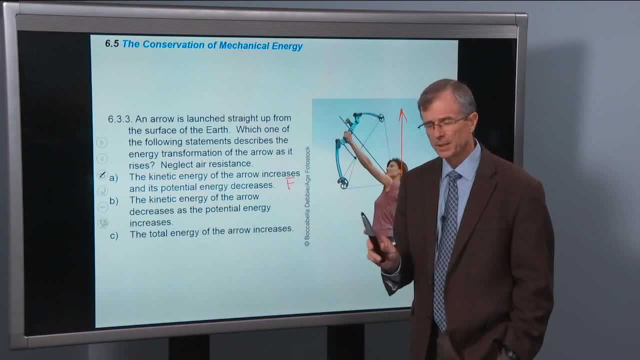 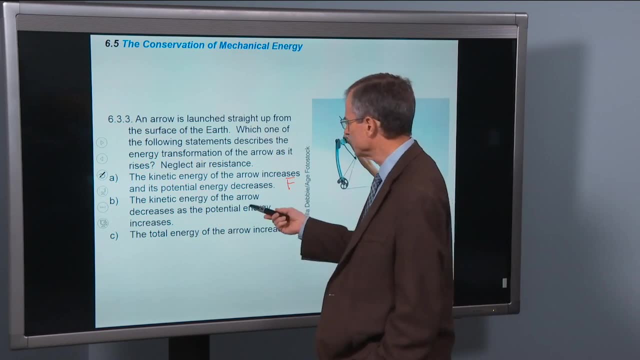 the potential energy increases, not the kinetic. The kinetic energy decreases because it's going to slow down, The speed is going to be less. The kinetic energy of the arrow increases and the potential energy increases, And that's the one that we want. 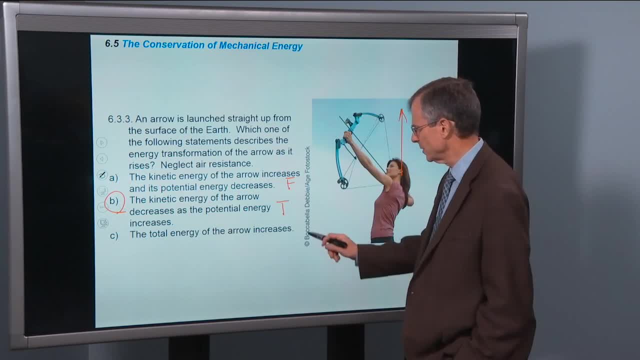 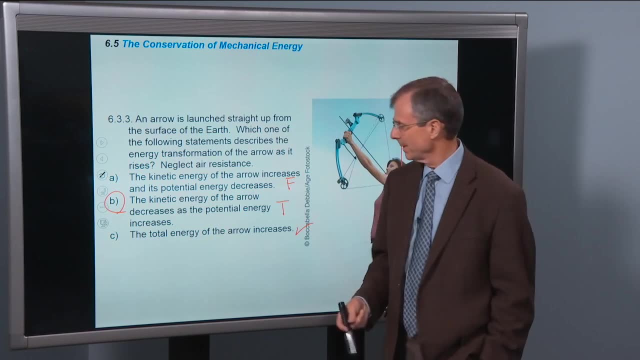 The total energy of the arrow increases. What about this one? The total mechanical energy, sometimes called the total energy and other times just called the energy increases. You say, well, no, that can't be. The energy would have to be conserved. 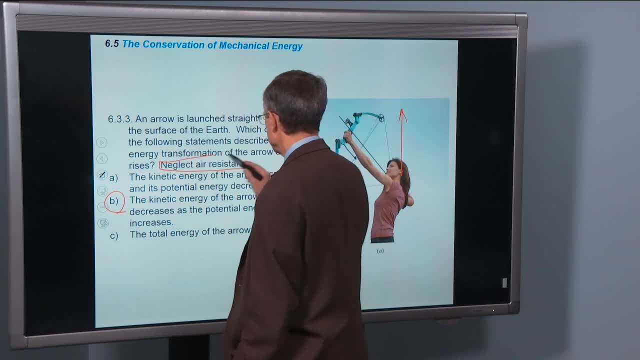 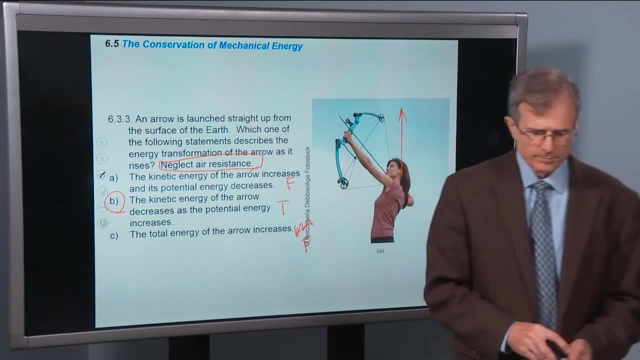 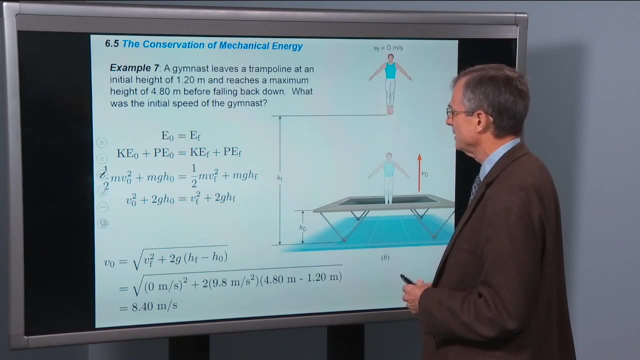 as long as we're neglecting air resistance, which would be a non-conservative force. So let's look at this one. Alright, a gymnast leaves a trampoline at an initial height of 1.2 meters and reaches a maximum height of 4.8 meters. 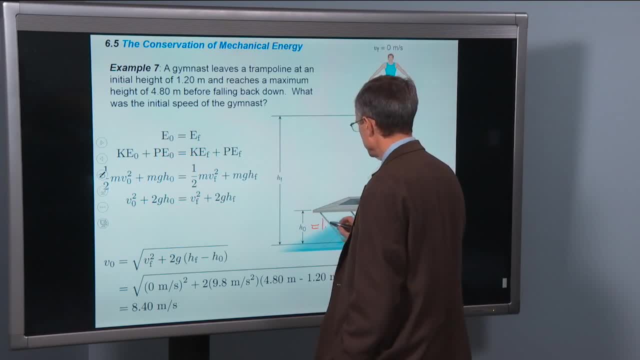 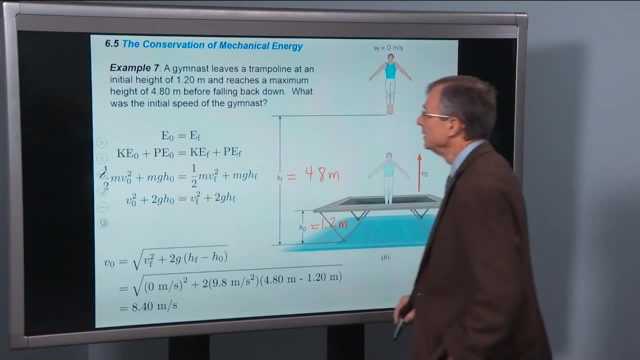 So this is: the initial height is 1.2 meters and the final height is 4.8 meters. Before falling back down, what was the initial speed of the gymnast? Great question. This is an example of the power of conservation of energy. 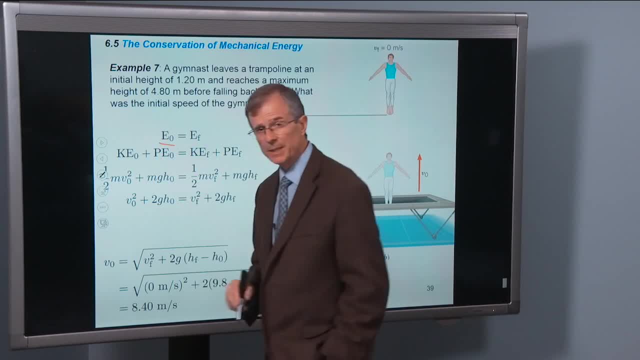 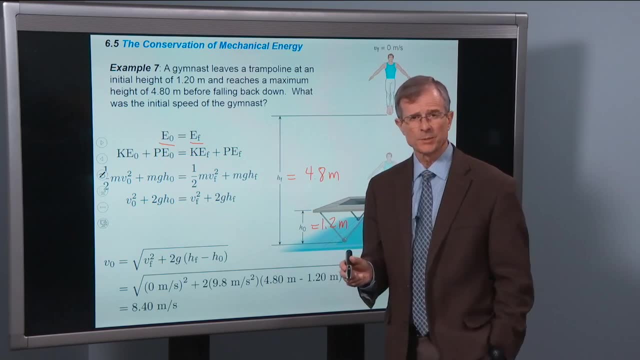 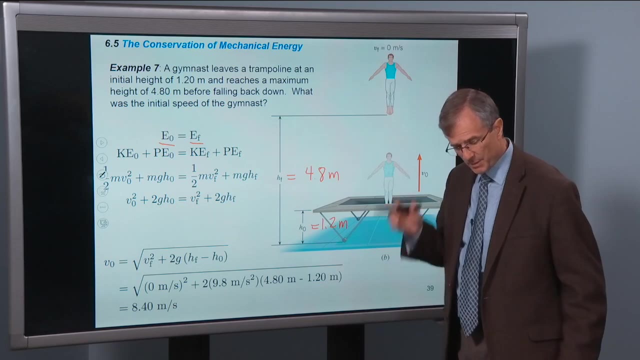 Let's do it. The initial total mechanical energy equals the final total mechanical energy. if non-conservative work done by non-conservative forces can be neglected, Can it be neglected in this case? Yeah, he's a big heavy gymnast. 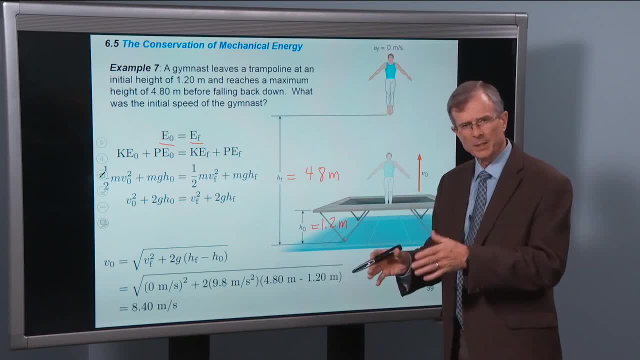 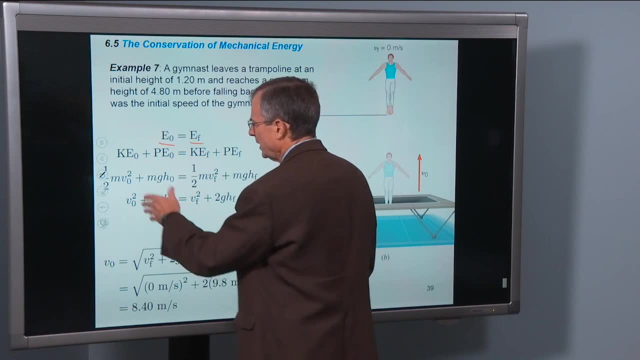 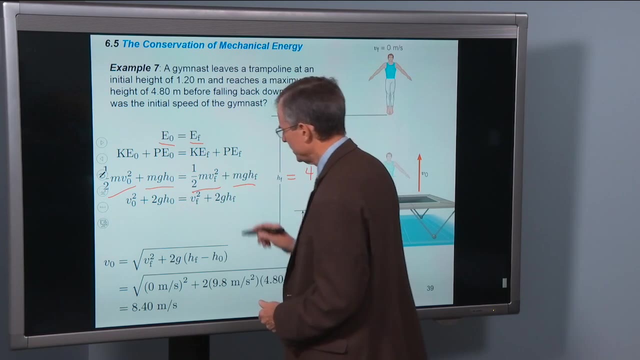 air resist. he's going to be moving fairly slowly through the air, so air resistance can be neglected In this case. initial kinetic plus potential: here's the initial kinetic, here's the initial potential energy, final kinetic, final potential energy. 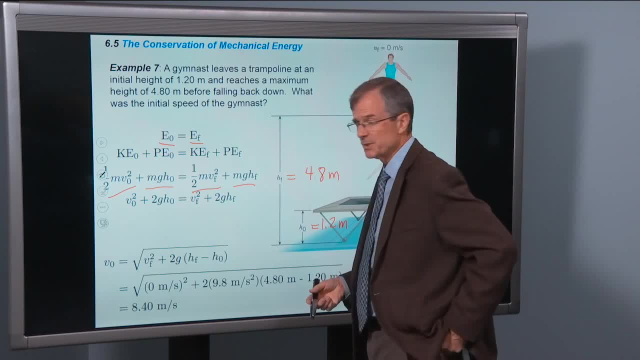 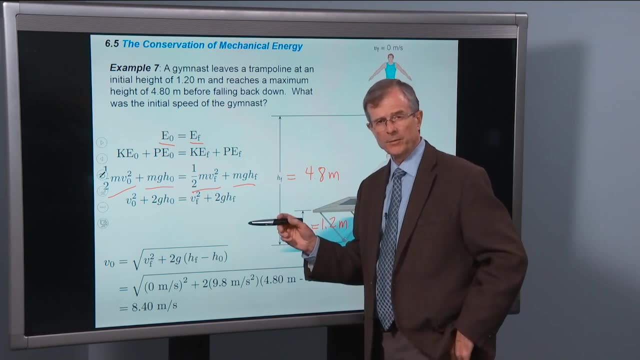 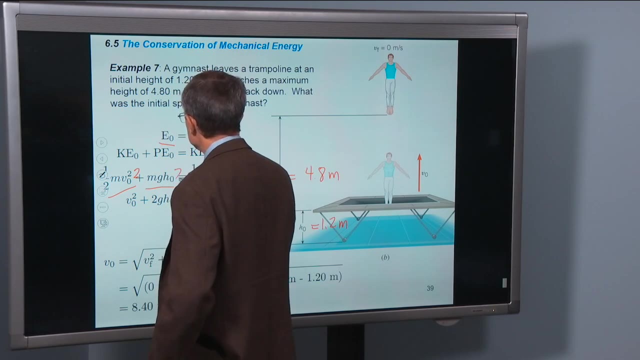 Let's plug. well, actually, what we're going to do is we're going to start cancelling some things. We can simplify this equation by multiplying through left and right sides by 2.. So I'm going to multiply this term by 2,, this term by 2,. 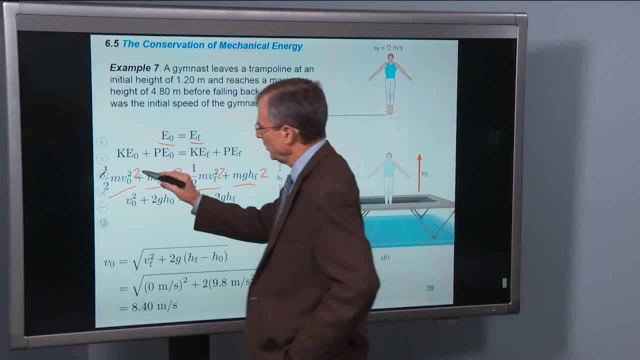 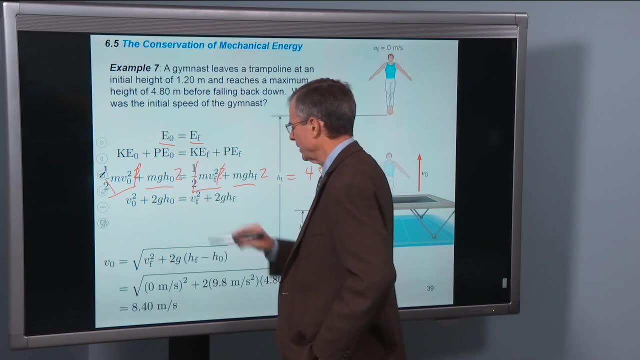 this term by 2, and this term by 2.. Well, that 2 cancels this 1 half. We'll have a 2 left over there. This 2 cancels that 1 half. Then I'm going to divide through. 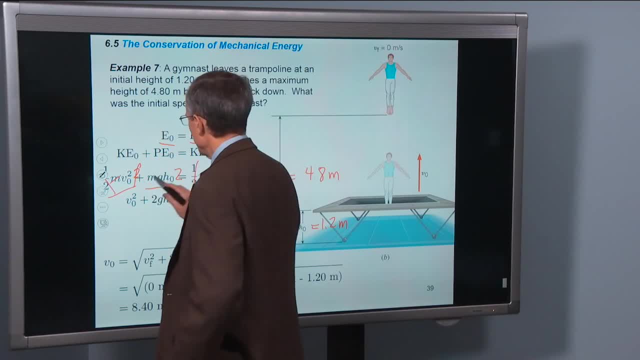 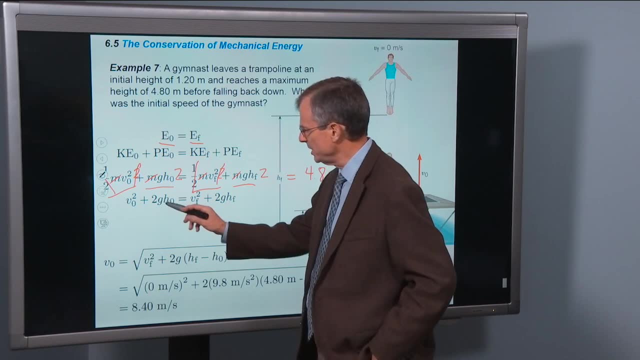 the whole equation by the mass, So that mass, all these masses, get killed And what's left over is V naught squared plus 2 G H naught. there's the 2, G H naught equals V F squared. 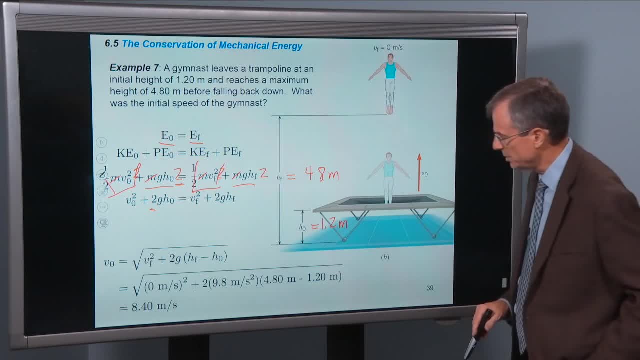 the final speed squared plus 2 G H and 2 G H final, We're looking for the initial speed of the gymnast. So it's an interesting thing. It's pretty easy to figure out. I mean, you can estimate. 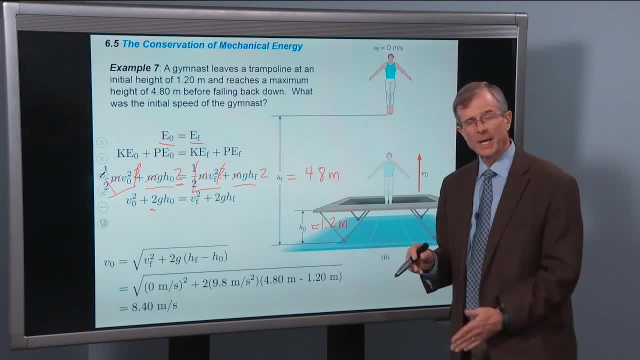 you can put a little ruler or tape measure, find out how high the gymnast went, and that's easy to measure- 4.8 meters- But it's a little harder to measure the velocity. This is an example of a problem where you can actually calculate the velocity. 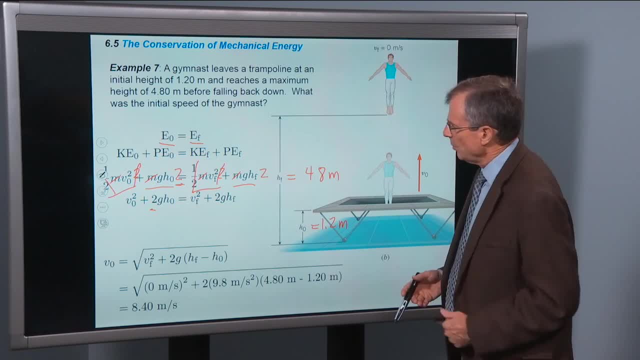 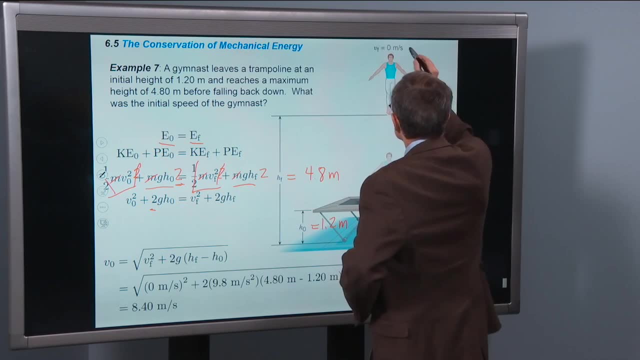 the initial velocity. Well, to find V naught, that's what we're looking for, his initial speed here. His final speed is 0. But to find the initial speed, I'm going to have to solve this equation for V naught. 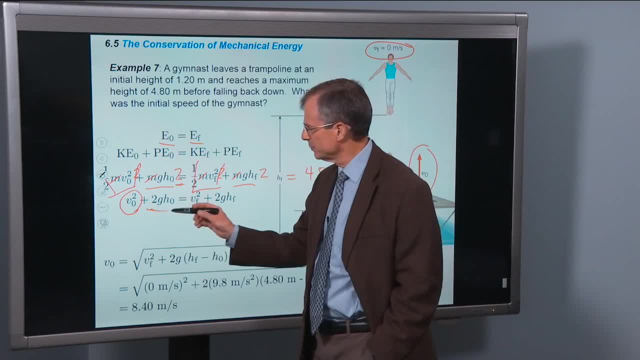 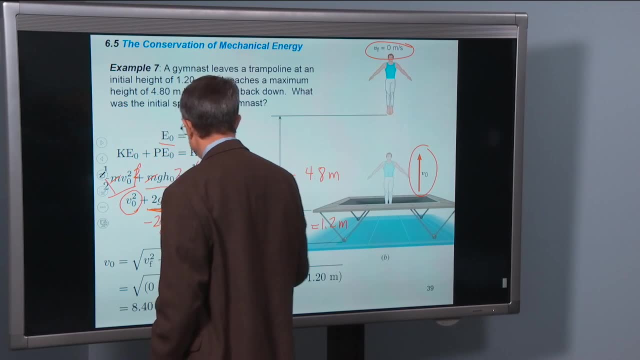 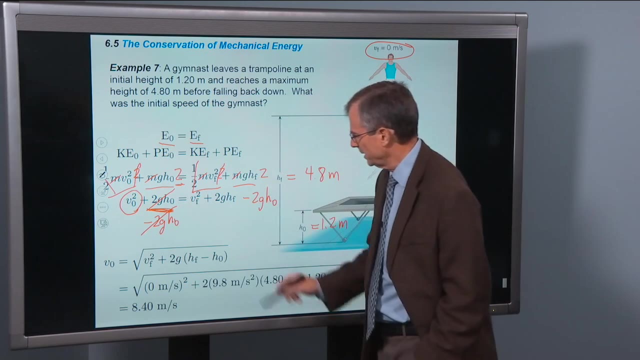 How do I do that? How about if we subtract 2, G, H, naught from both sides of the equation? It'll cancel on the left side and we'll be left with this mess on the right side. Then we're going to take the square root. 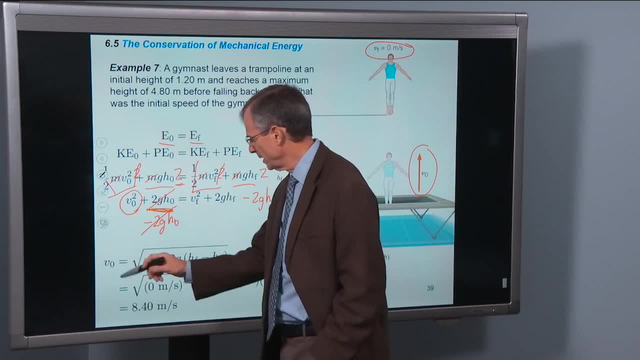 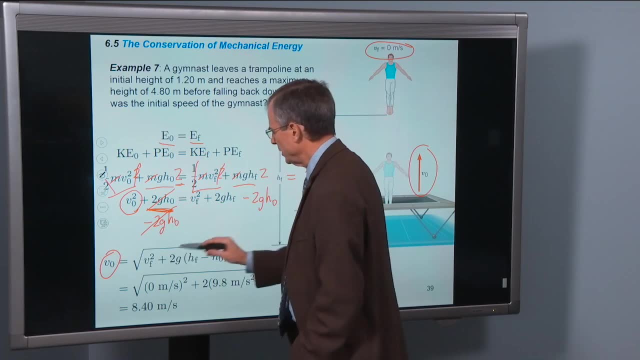 of V naught squared to find V naught. And here we go, Here's my V naught, and I had to take the square root of this whole mass, the square root of V F squared. that's that term 2 G, H, F is this term. 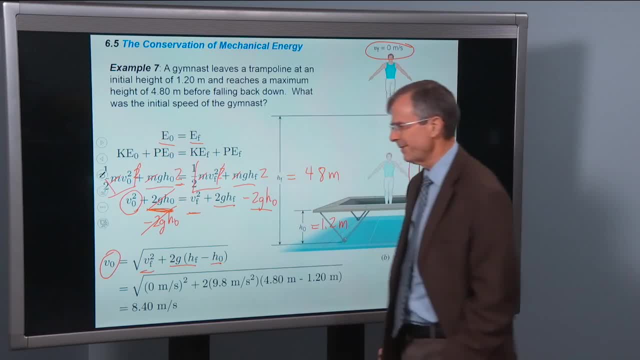 2 G H. naught is that term where I've factored out the 2 G. Well, now we can just plug in the numbers. We know that the final speed is 0 meters per second, and we know 2,. we know G. 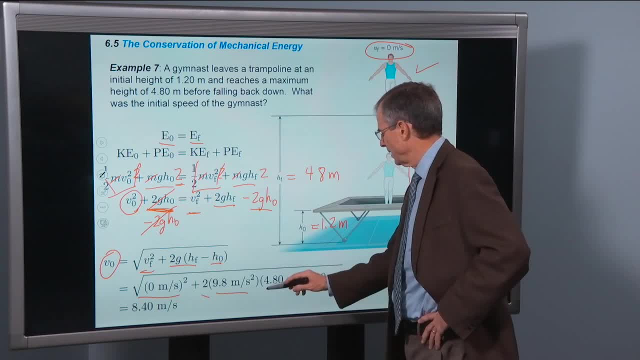 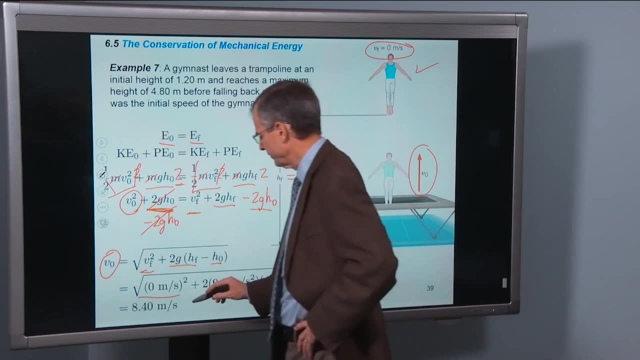 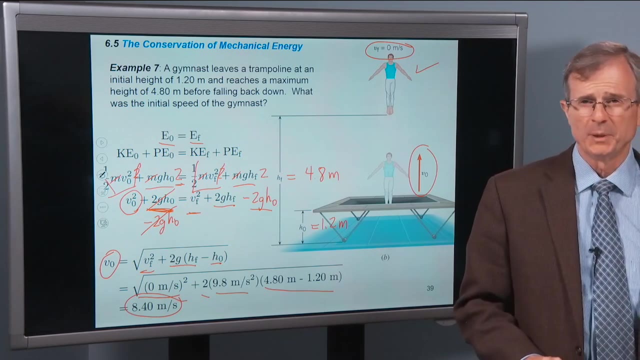 gravitational acceleration, final minus initial heights, And we plug the numbers in and you get 8 and a half, roughly 8 and a half meters per second. That's how fast he was going when he just left the trampoline mat. Another example: 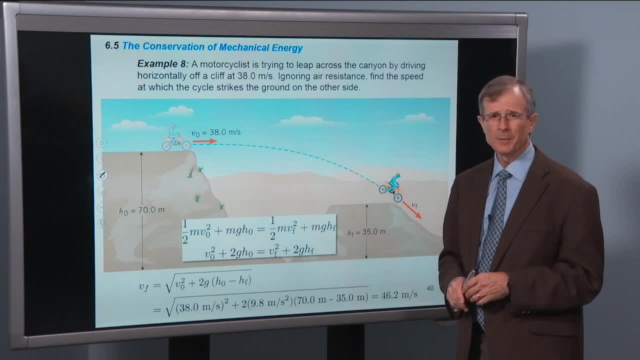 It's actually similar in a lot of ways, but it seems a lot more complicated. This one seems really bizarrely hard, but it's very easy with conservation of energy. A motorcyclist is trying to leap across a canyon. this is Evel Knievel. 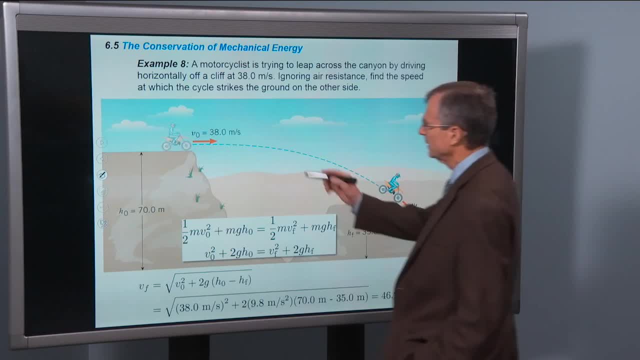 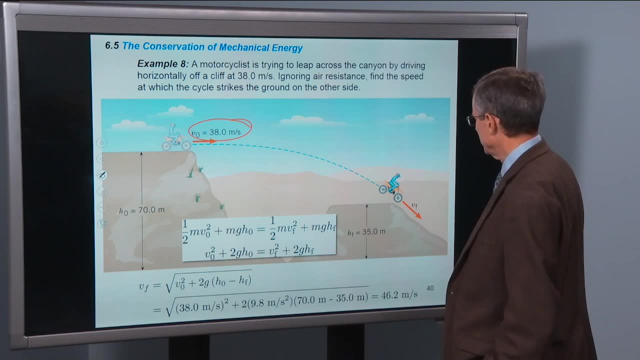 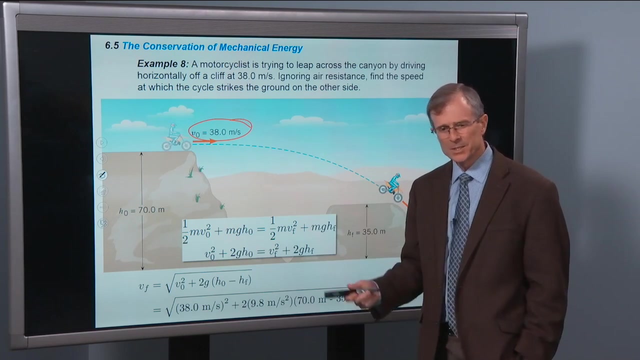 by driving horizontally off a cliff at 38 meters per second, Ignoring air resistance, find the speed at which the cycle strikes the ground on the other side. As long as you don't need the time of flight, then conservation of energy is going to be your friend. 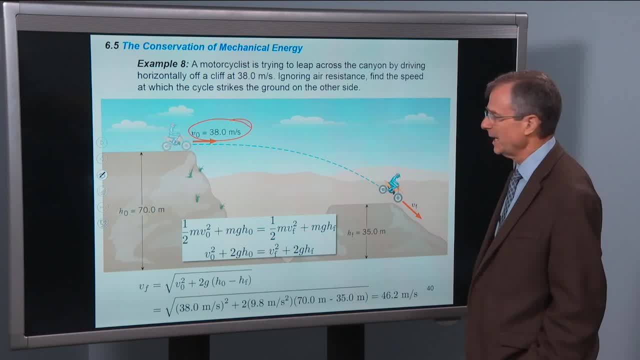 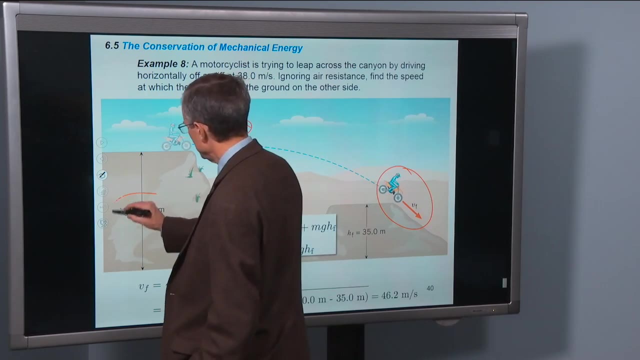 for solving problems. In this case, they're not asking how long he was in the air. all we're trying to find is his speed when his cycle strikes the ground. on the other side, The diagram shows that his initial height is 70 meters. 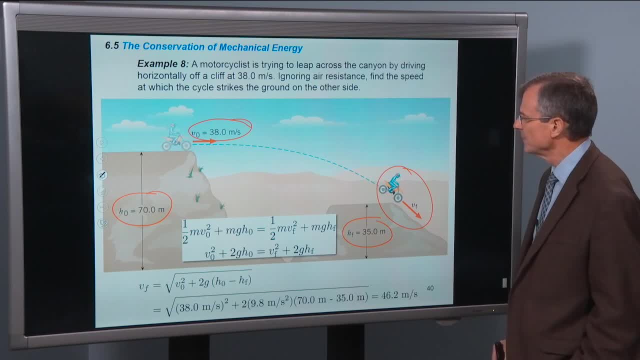 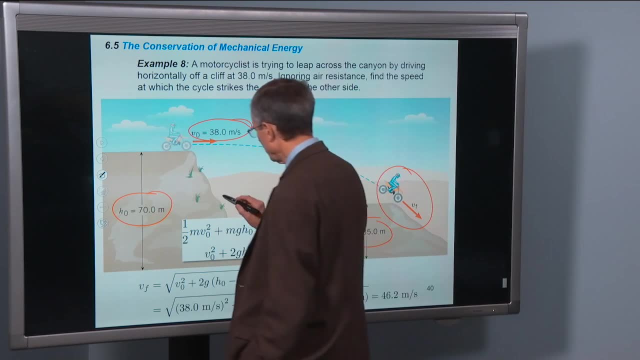 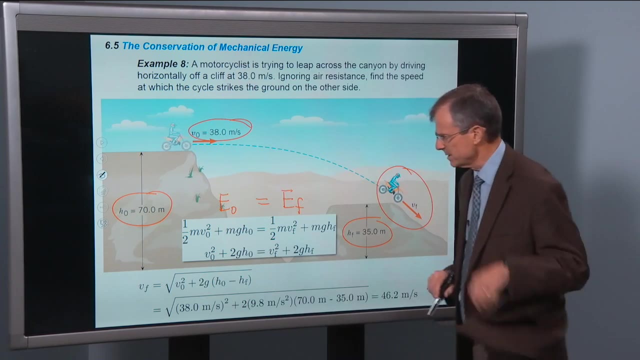 His final height is 35 meters, And so we can now apply conservation of energy to try and solve the problem. Here's the initial total mechanical energy on the left side, and here's the final total mechanical energy on the right side: Kinetic plus potential. 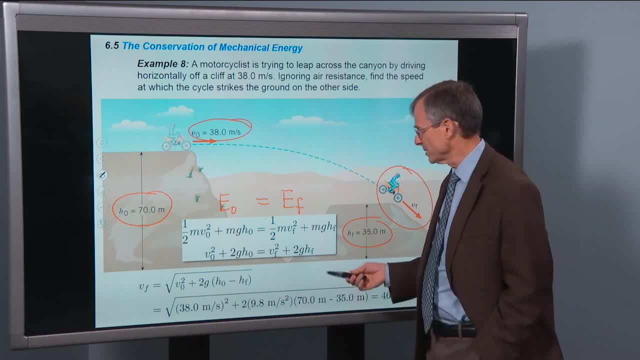 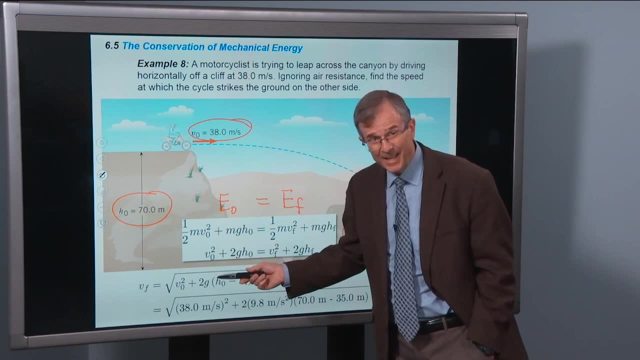 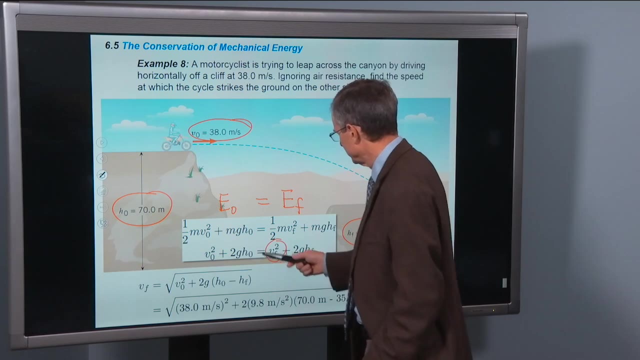 We multiply through by 2, divide by mass. same as we did in the previous one, get this equation. Instead of solving for v naught now we're going to solve for v final because we have v naught, So we solve this equation for v final. 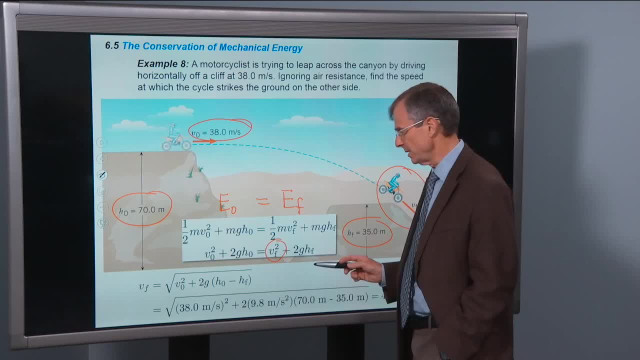 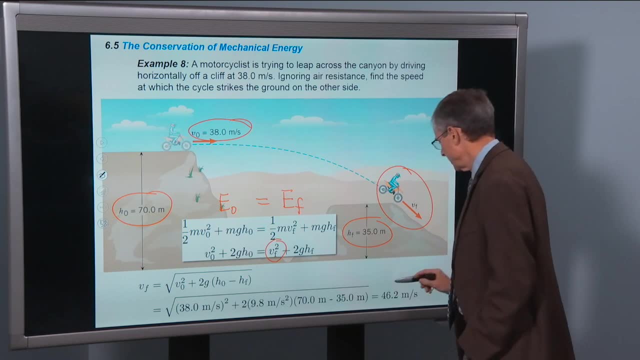 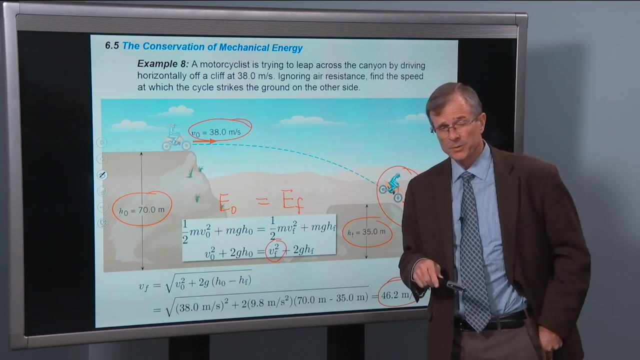 by subtracting 2ghf from both sides of the equation, giving this result: the algebra is similar to the last example. plug in the numbers and that gives 46.2 meters per second. Now for you to do this with chapter 3,. 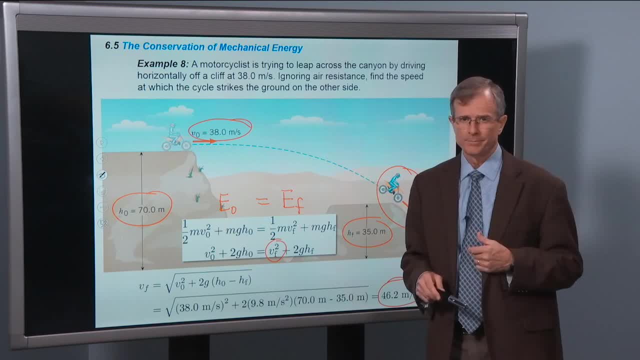 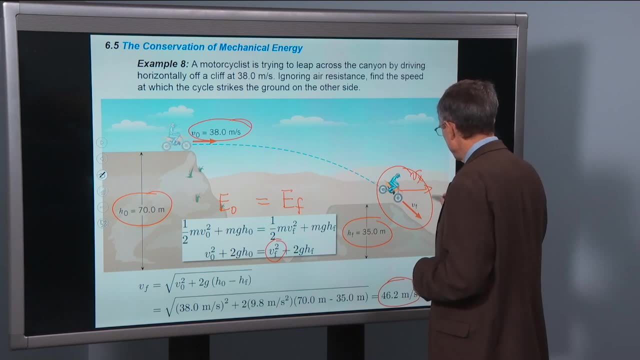 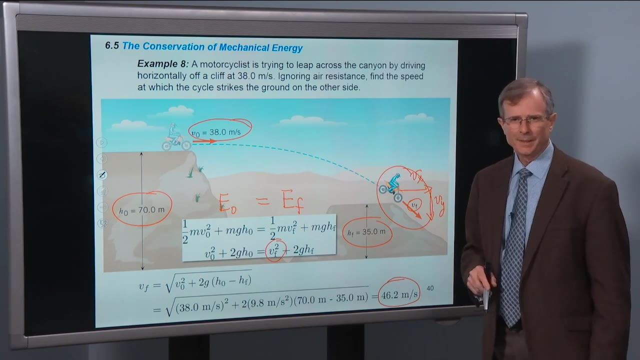 with the equations of kinematics would have taken you a long time, And the reason is you would have had to find the x component of final velocity, the y component of final velocity. you would have had to find the final speed by the square root of the sum of the squares. 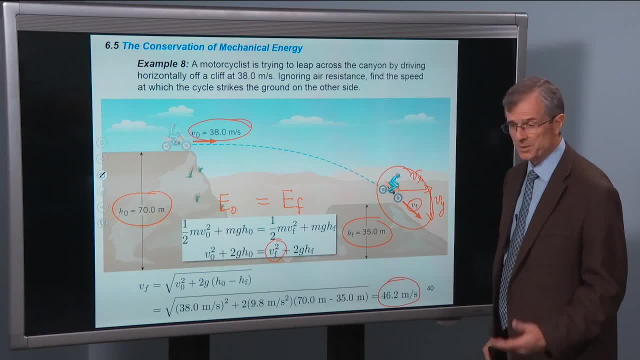 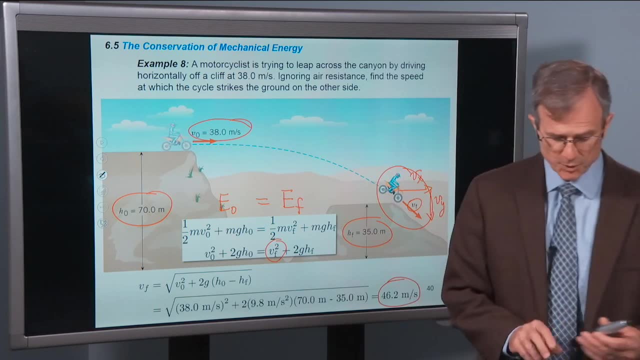 of the components of the speed, of the components of the velocity, and it would have been a big amount of work. This is just essentially a step or two of algebra. As long as you can do this algebra, you'll be great. What about this one? 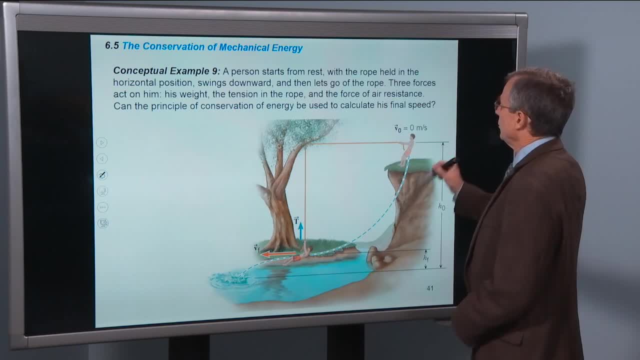 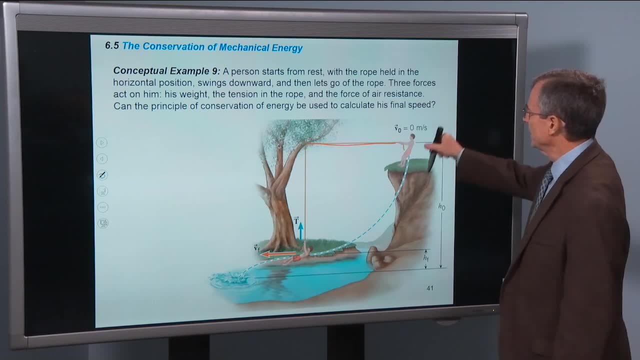 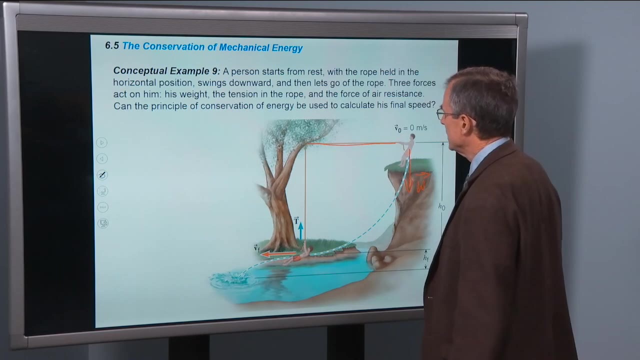 A person starts from rest with the rope held in the horizontal position. So here's: the rope Swings downward and then lets go of the rope. Three forces act on him: His weight, the tension in the rope and the force of air resistance. 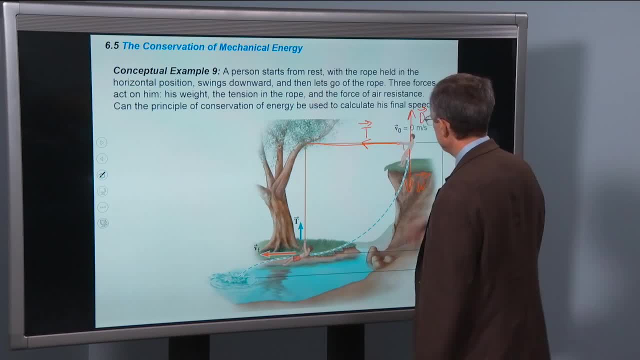 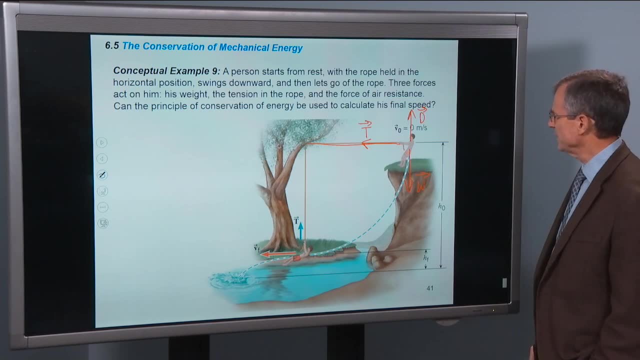 So there might be some drag here. Let's just call it with a D. Can the principle of conservation of energy be used to calculate his final speed? The short answer is yes. The tension is a non-conservative force. It was on the list of non-conservative forces. 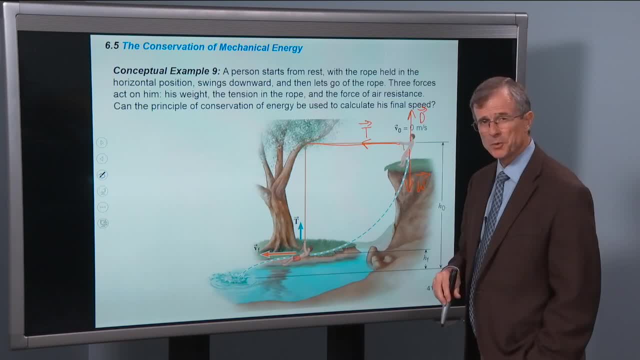 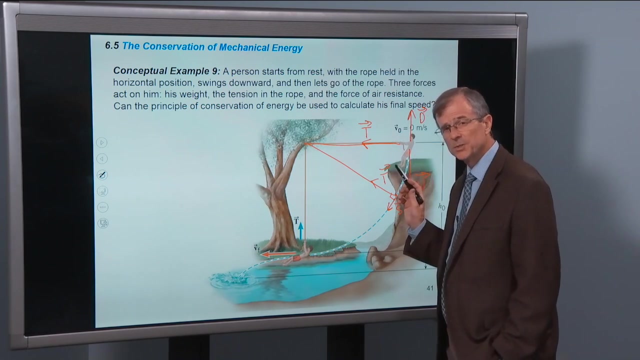 However, the tension does not work. Why His displacement at any given point? let's look at this point here. His displacement is this way, The tension is that way. They are perpendicular to each other at all times, So the work done by tension can be neglected. 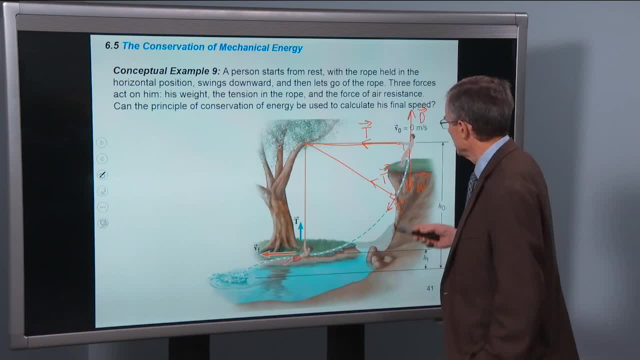 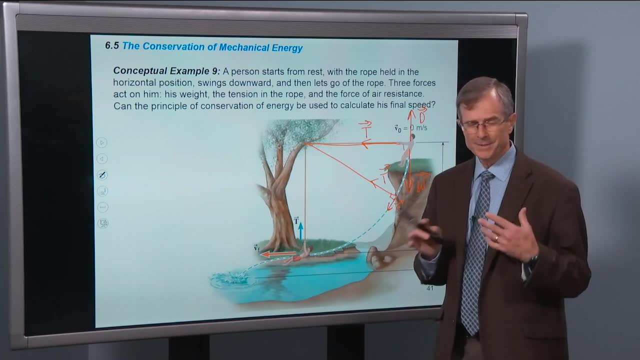 It's negligible. What about the work done by air drag? Well, he's a heavy guy. He's not going very fast. I know these arguments are a little bit hand-wavy, but if you've got a person that's moving at normal speeds, 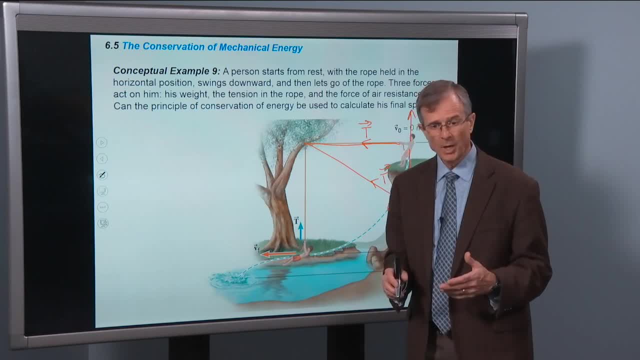 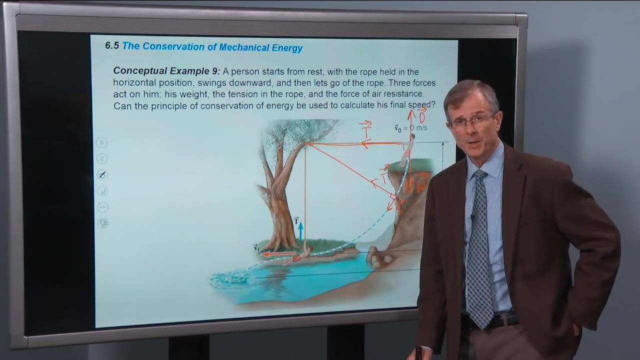 speeds that you can run or walk or swing on a swing. usually the air resistance can be neglected. As soon as you're getting up to sprinter speeds, with sprinters running 15 miles an hour or something like that, then air drag might become important. 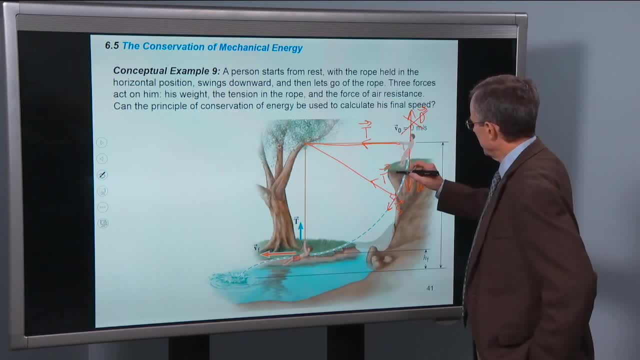 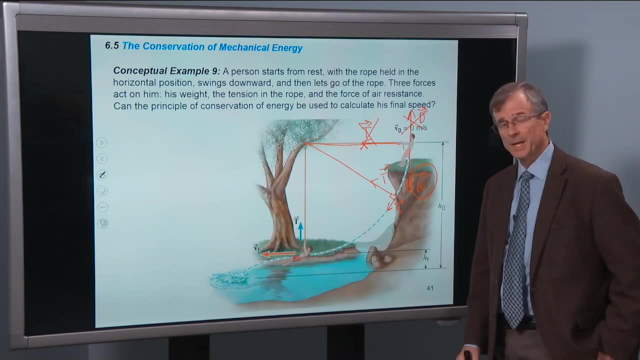 So this can be neglected: The work done by the air drag, the work done by tension, and we only have the work done by gravity, And that is conservative force. So we can actually use this to calculate his final speed, And this one will be exactly the same. 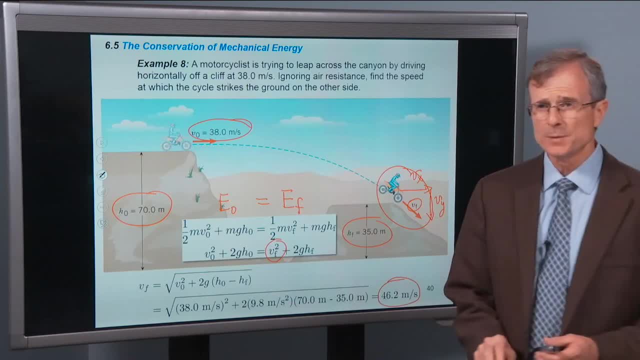 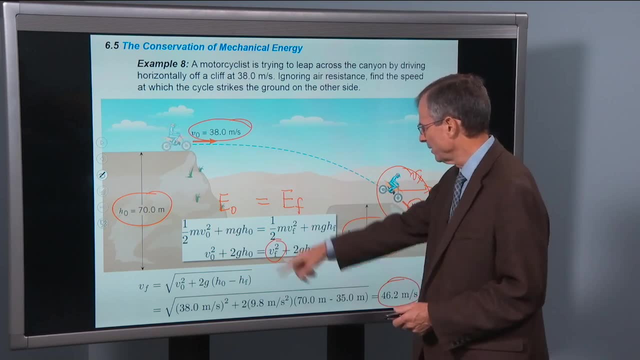 We do the algebra exactly the same as you did for this motorcycle: You have an initial speed here, and then you have an initial speed here, and then you solve this equation to find his final speed Here it's even easier because the initial speed is zero. 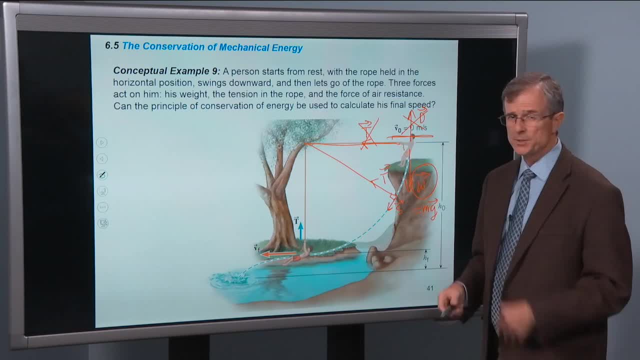 So you just use that same equation and plug in the numbers that you have and you'll find I guess you'll need the radius of this rope. It's not given to us, but we can certainly. if you knew that, then you could do the calculation.